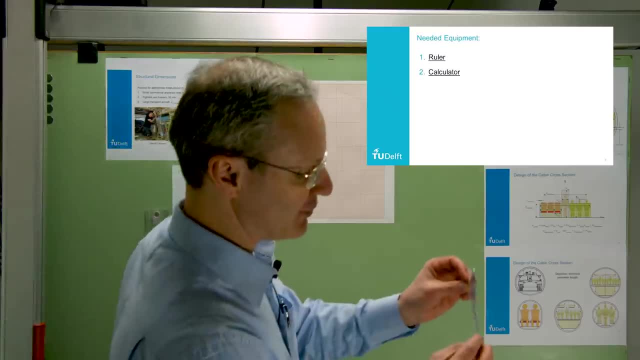 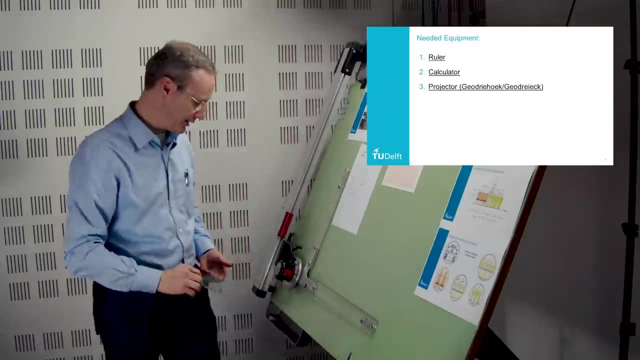 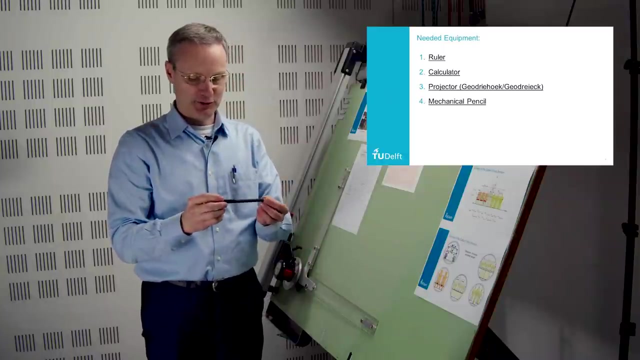 calculate a couple of things. We have this little device which is called a projector, or in Dutch, Geodriehoek. It costs about 50 cents and it's a very handy tool. You definitely must buy one. Then we have a refillable pencil. This is one which has a diameter of 0.5 millimeters. You 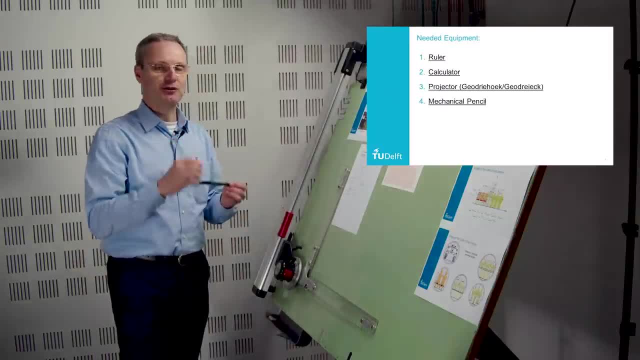 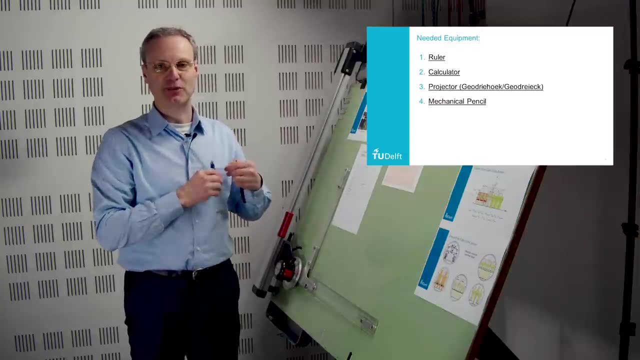 have to be careful with that. If you're a bit more sturdy in using your pencils, you can go to a bit thicker one- This is a 0.7 millimeter pencil- but then the lines become thicker and the drawing becomes less accurate. 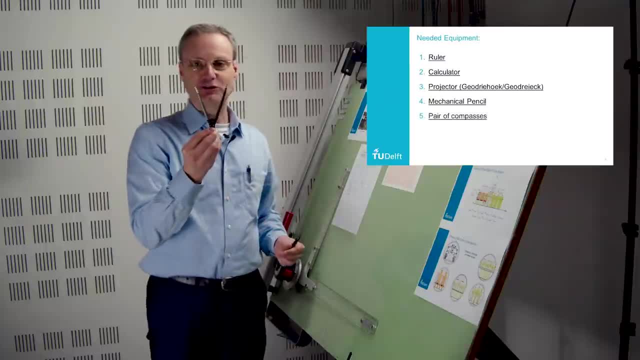 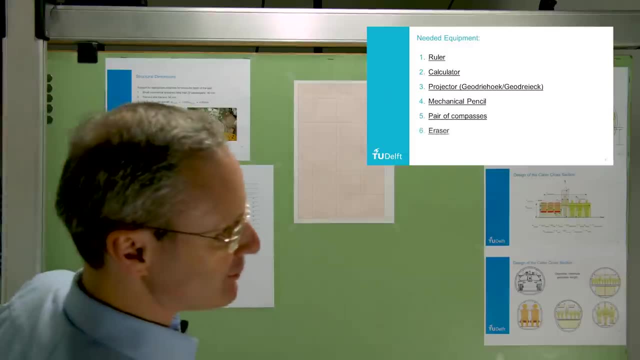 And of course, we need a compass. This is not a naval compass, but this is one just to draw circles And of course, it's possible that you make mistakes. Also, an eraser is very handy. So that's the tools we're going to use today. 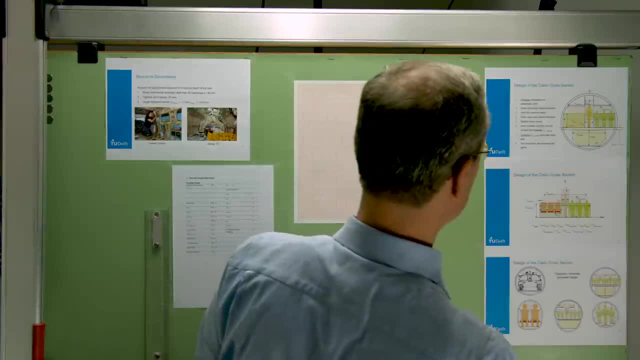 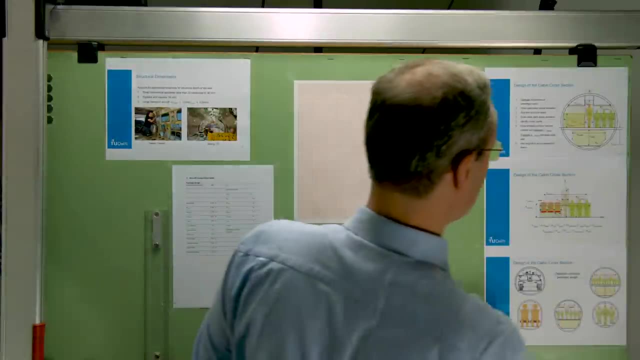 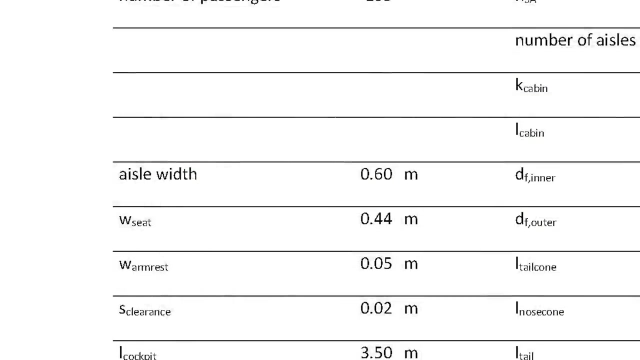 So let's make a start. First step: compute the dimensions. What we have already been given is the aisle width here, So we can put that into the, into the formula. We have 0.6 meters for the aisle width, We have the width of the seat, And then, of course, you can say: 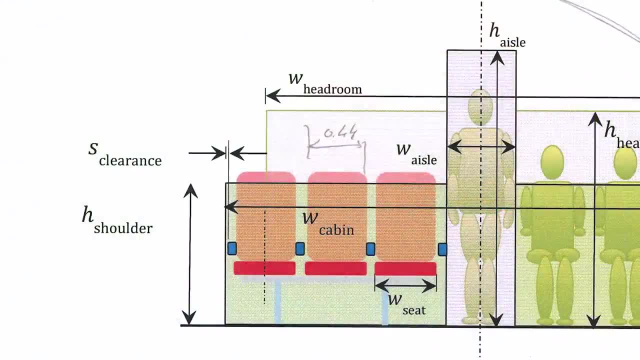 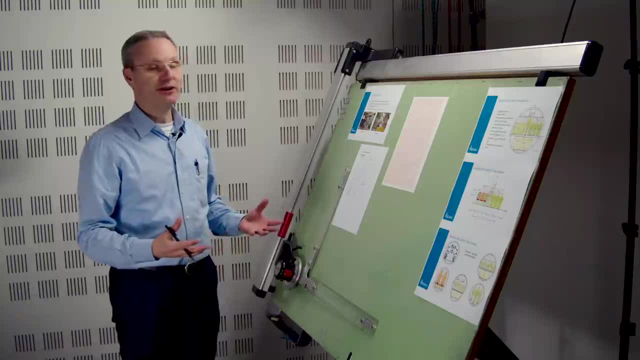 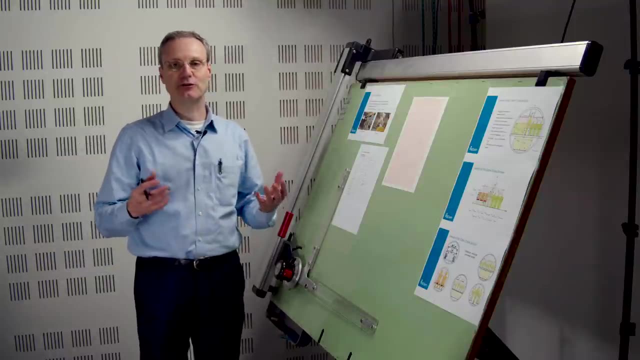 okay, this one individual seat which that we have here has a width of .44 millimeters, 44 centimeters, But we need to know how many seats we have. So to determine how we have, we first need to calculate the amount of seats abreast. So that's. 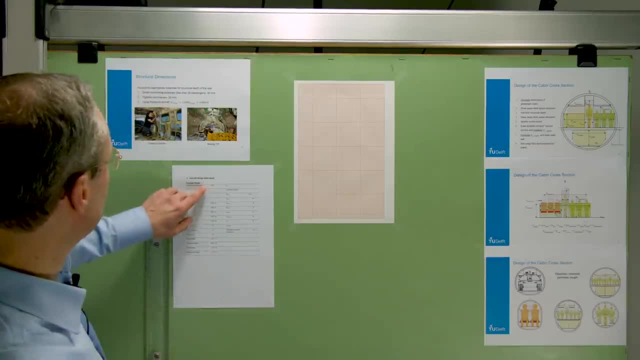 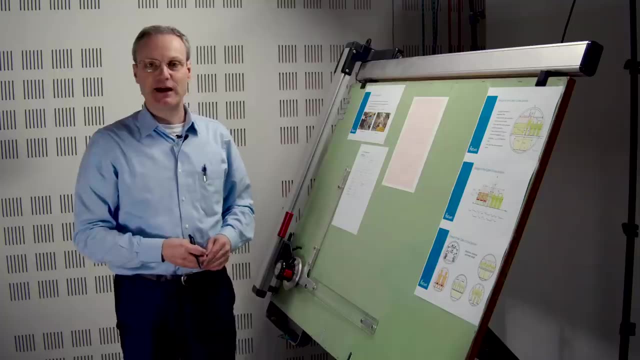 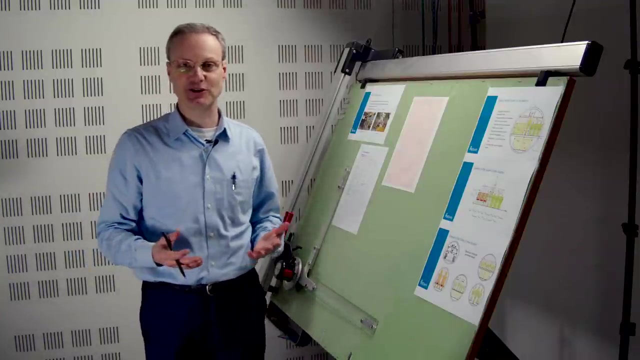 where we're going to do a first calculation. What we need to do is take a look at the number of passengers, plug that number into the formula- there's this formula with the square root- and then you'll figure out that the seats abreast is a little over four and a half. Well, we don't put half passengers in the 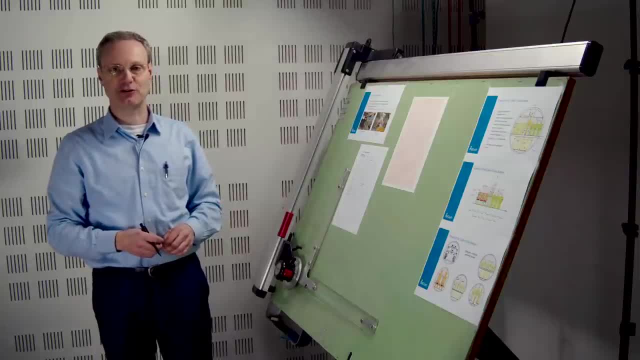 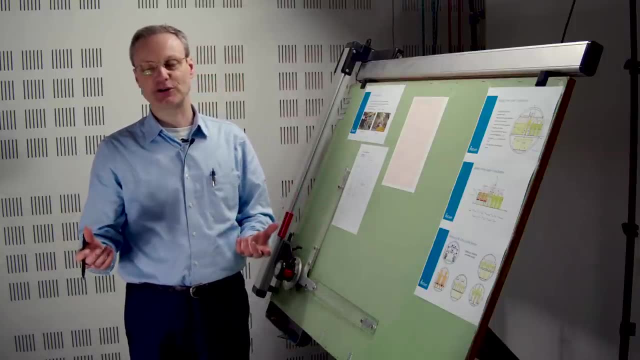 seat, so we round that up to five seats abreast. So in total we will have five seats abreast. This is an aircraft which has less than six seats abreast. that means we have one aisle only. so we have one aisle only, one aisle that we'll take. 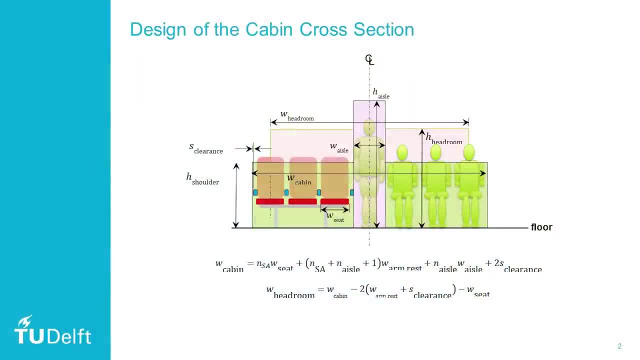 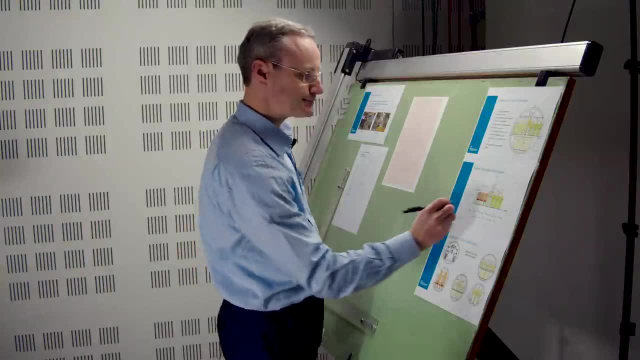 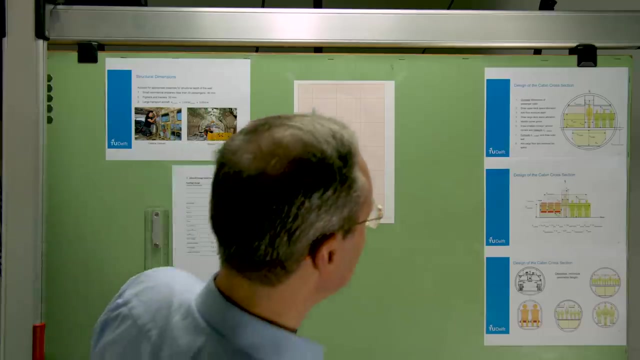 into account, but we have five seats. So we have five seats. number, five seats abreast times the width of the seat: 0.44 millimeters. Then we have of course to take into account the room for the armrest. we will have the number. 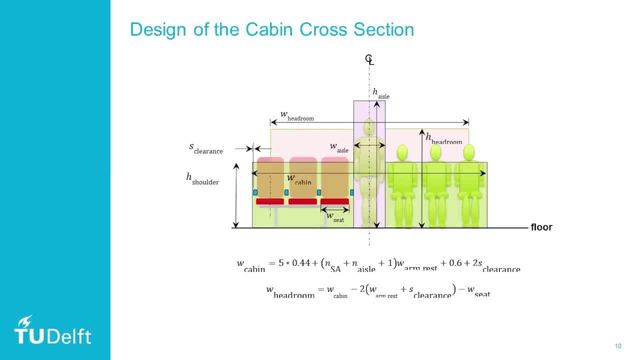 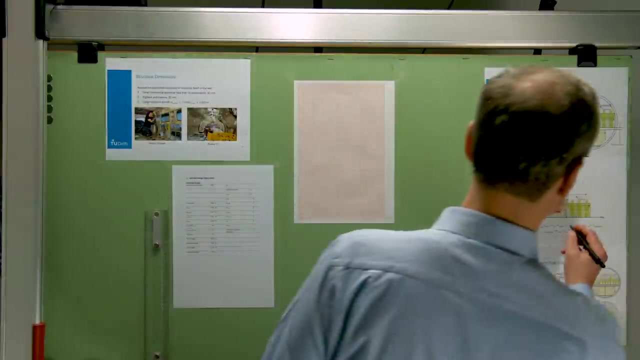 of seats plus the number of aisles, plus one armrest, So we have five plus one is six plus one is seven, Seven multiplied by the armrest, and the data for the armrest has been given as 0.05 meters, so five centimeters. so multiplied by 0.05.. 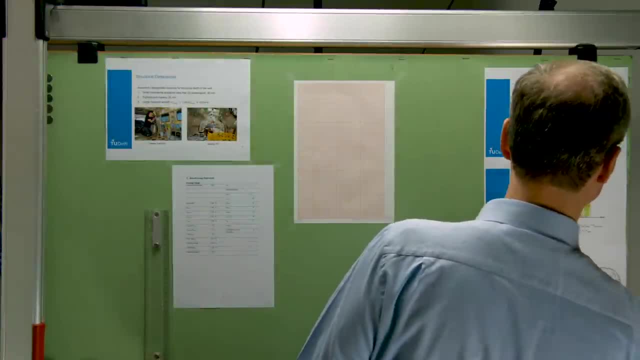 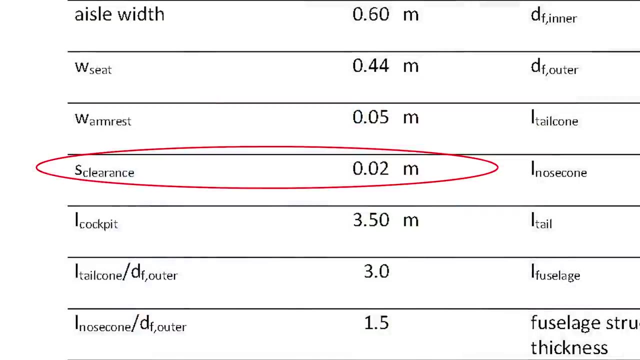 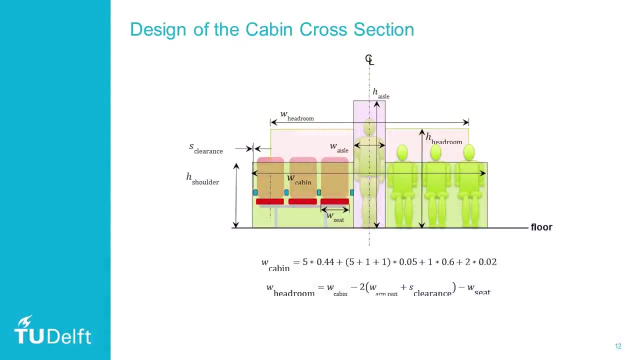 We have one aisle. that's what we already calculated, multiplied by the aisle width of 60 centimeters, and then we need two times the clearance, and the clearance has already been given as two centimeters. so plus two times 0.02. 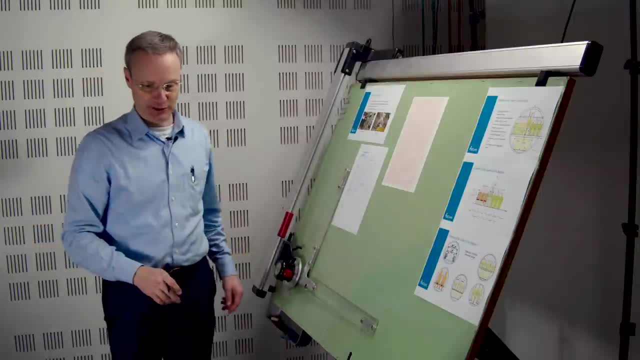 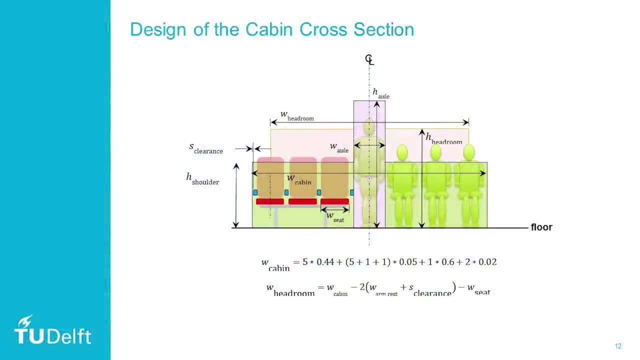 meters, And then we have all the elements for the width of the cabin, and then we can start out drawing. So let's see what we have: Five times 0.44 meters plus seven times 0.05 meters plus one time the aisle: 0.6 meters plus two times. 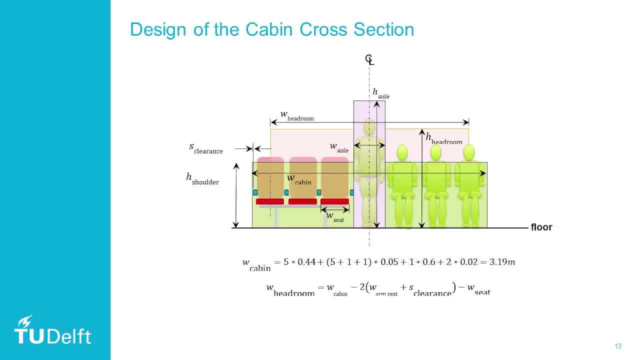 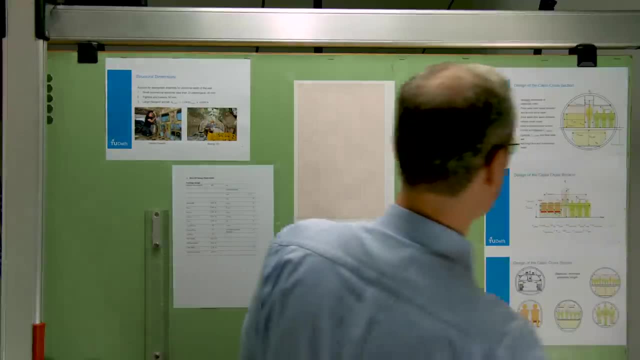 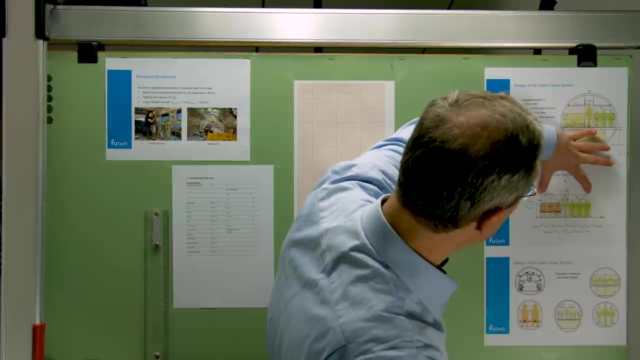 0.02 meters. It's 3.19 meters, so this one is 3.19 meters. Then we need to find the headroom. The headroom is this width here, the width at the headroom, So we will have a. 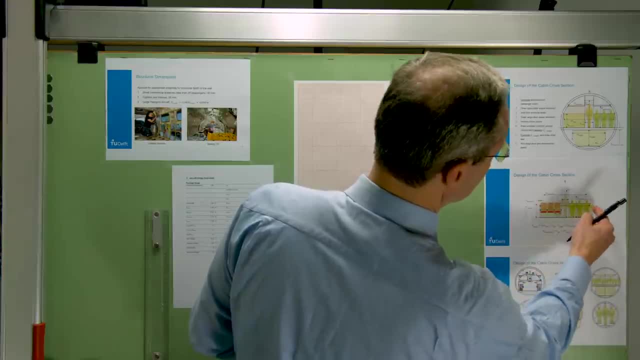 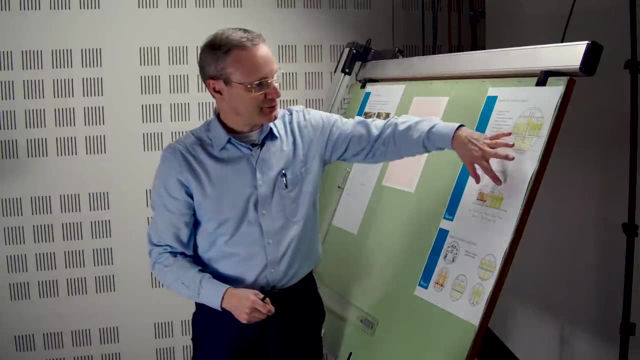 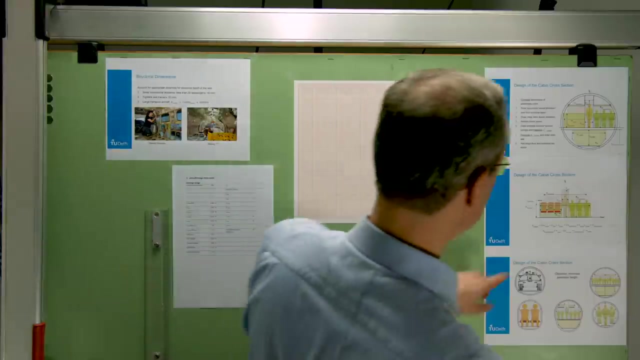 fuselage, which will be looking like this, and, of course, the space available will become less if we start from the widest point, And we need to find out how much space we really need here, because this will be one of the corner points in the design. So let's do that. The headroom is given as the width of the 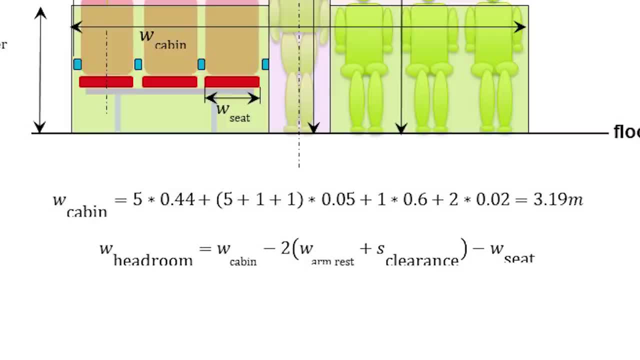 cabin. We just calculate that as 1.39 meters minus two times the width of the armrest. The armrest we get from the, the graph again from the table, again five centimeters plus one time. the clearance was two centimeters, 0.02, close. 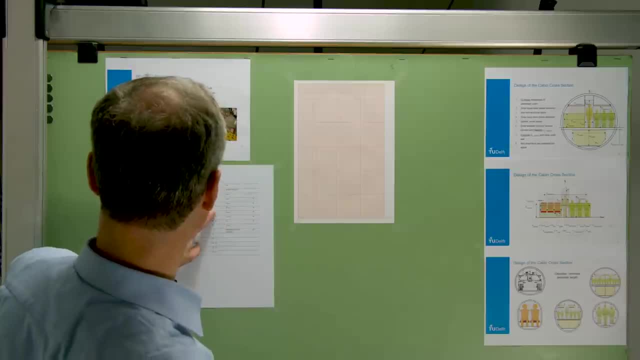 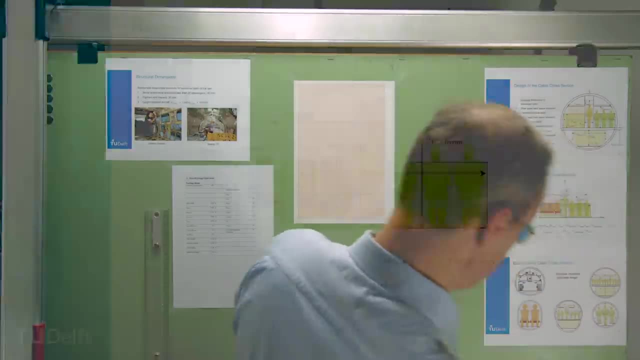 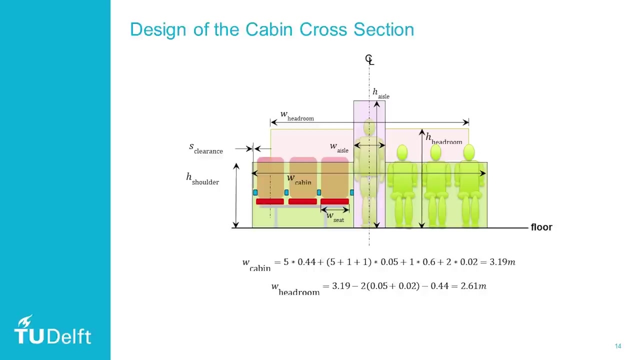 bracket minus the width of the seat, and the width of the seat we already used before, 44 centimeters, 0.44 meters. Make the calculation again, So what we will see is that we have 3.19 minus 2 times open bracket, 0.05 plus 0.02, close. 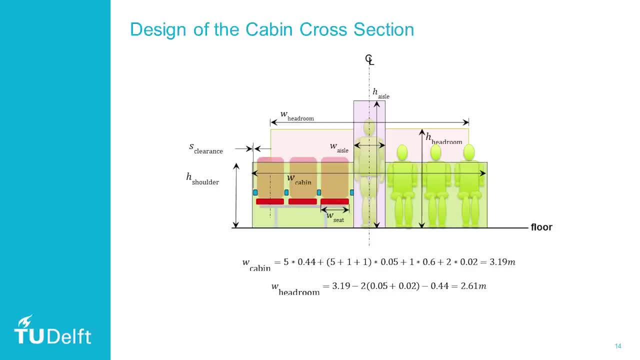 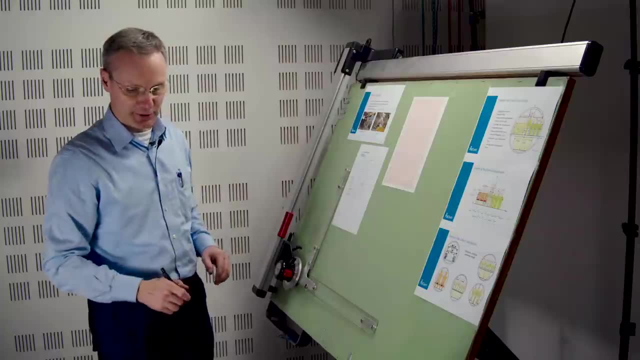 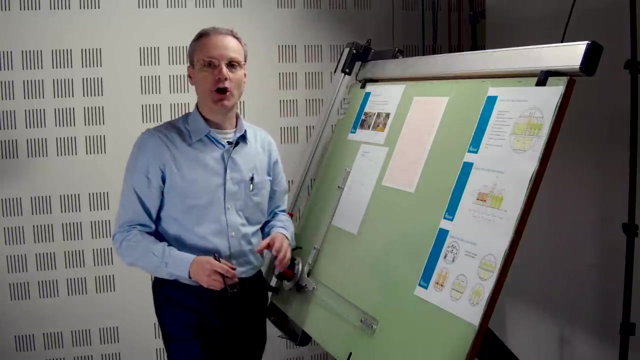 bracket minus 0.44.. That's 2.61 meters. So we have some principal dimensions. Okay, that means that we can now start our drawing and since we don't know where the center line is going to be- because we have an odd number of seats- we cannot. 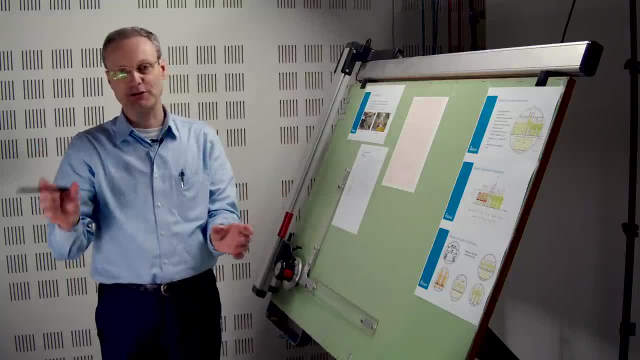 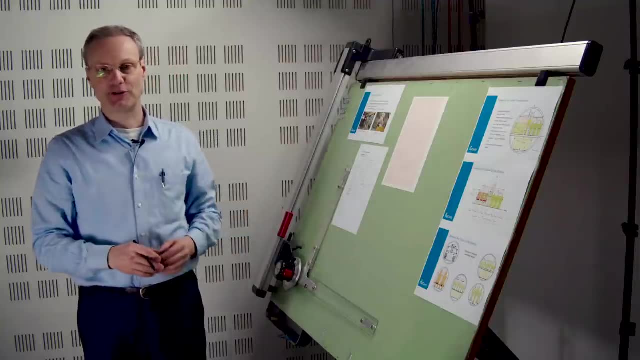 split them: two on the left-hand side, two on the right-hand side. that's four breast or three, three. we have five seats of breast, So it's going to be a 3 plus 2 split. so the aisle will not be in the center. 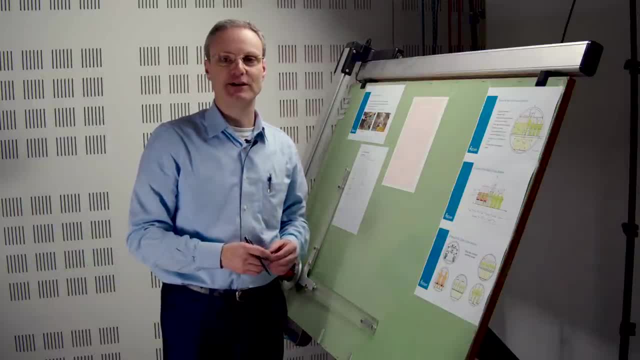 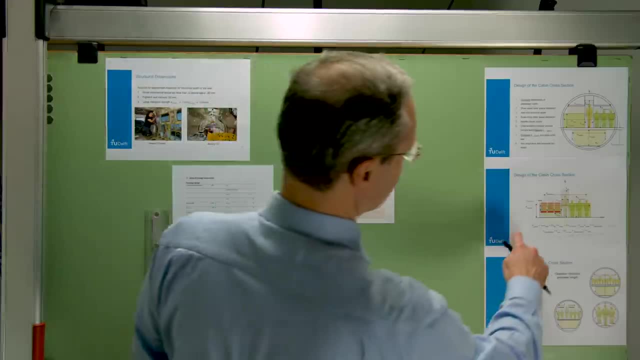 line. So that means you will not be able to draw the vertical center line of the fuselage yet. We will do that later on. So what we'll do in this case? we'll start by giving the floor, so we'll draw the floor. I can do that with this. 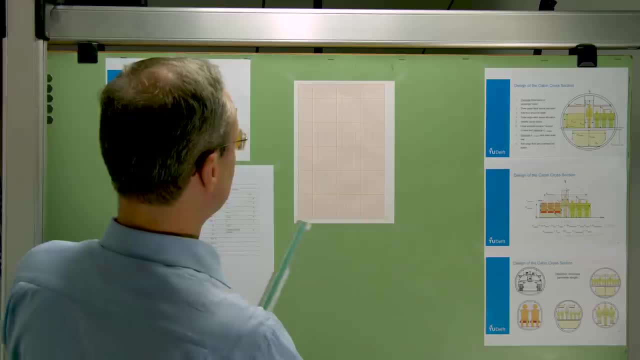 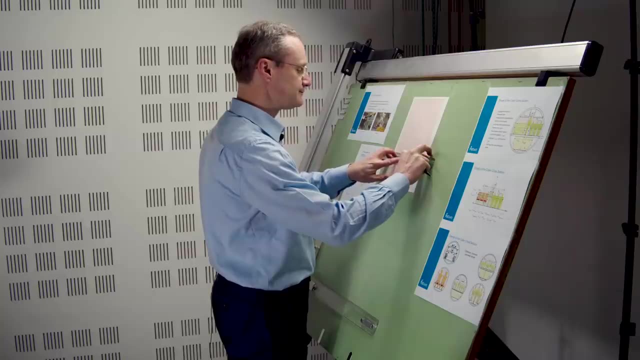 machine. of course that's an easy one, but I'll do it like you will be doing, just with my ruler, and I'll just set the floor somewhere on my drawing, Make a nice straight line, do it a bit below the middle of your picture. 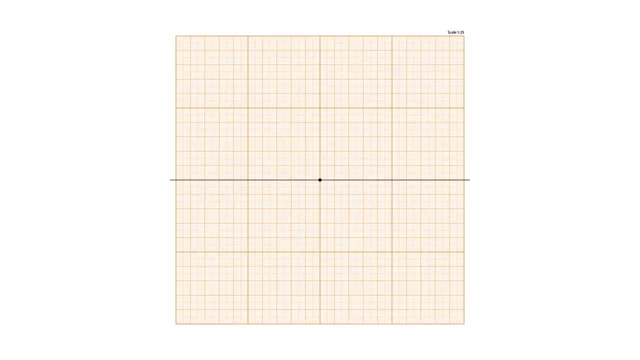 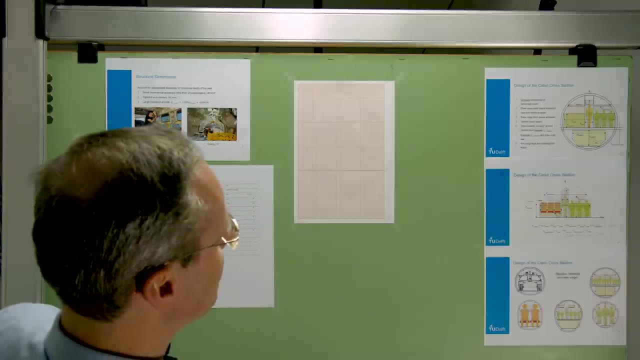 put it on a square tarpon and draw a nice straight line. so that's going to be my floor. I'll just write it here so we know what we're talking about. and now what we're going to do. we're going to define all these blocks, all these. 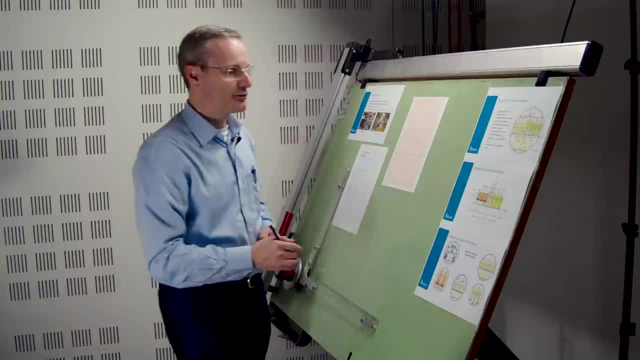 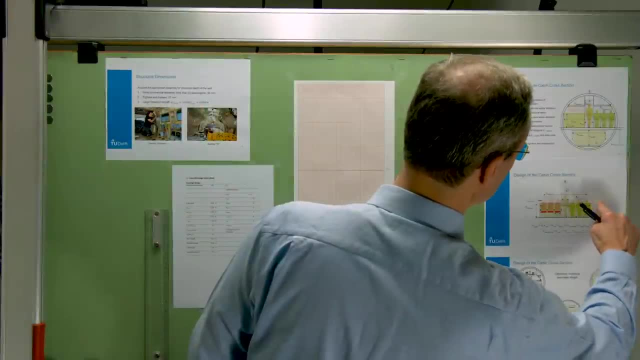 rectangles on the basis of the data we have so far. So the first one is that we will have a shoulder height that will be the height of the block. so I would want to draw this line here and the shoulder height has been given. 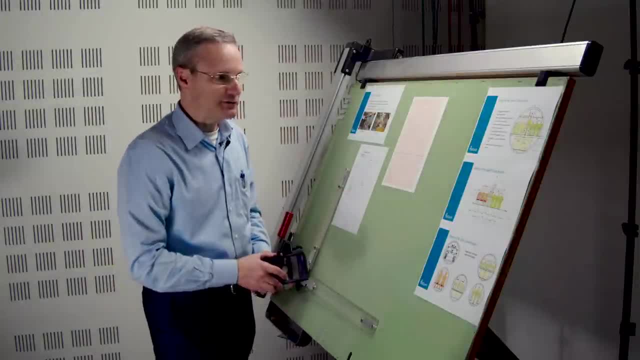 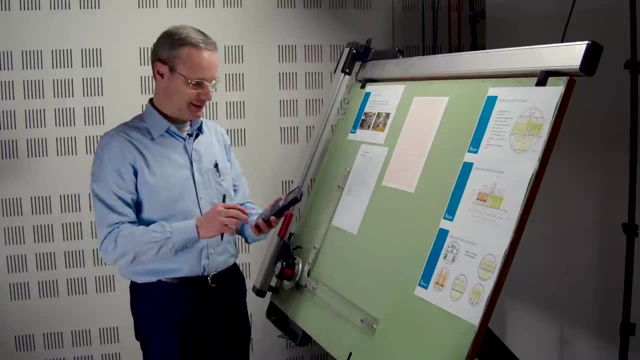 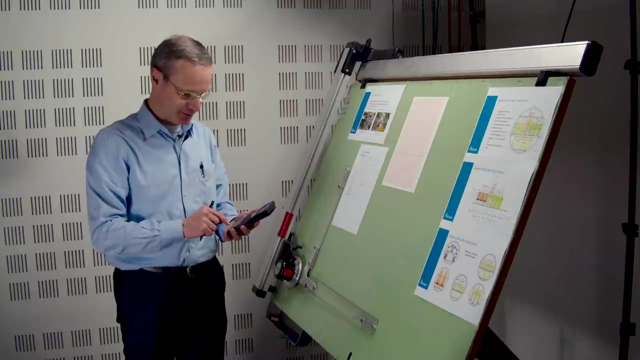 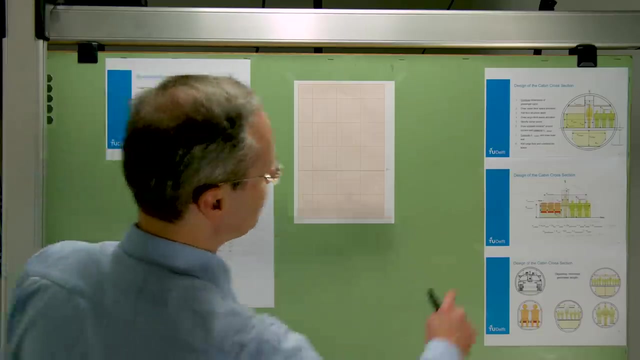 95 cm. Now, 95 cm has to be converted into the scale of this drawing And the assignment of this exam set a scale 1 to 25 scaling. So I have 95 cm and divide that by 25.. That means 3.8 cm or 38 mm. So that line, this line that I'm going to draw here, is going 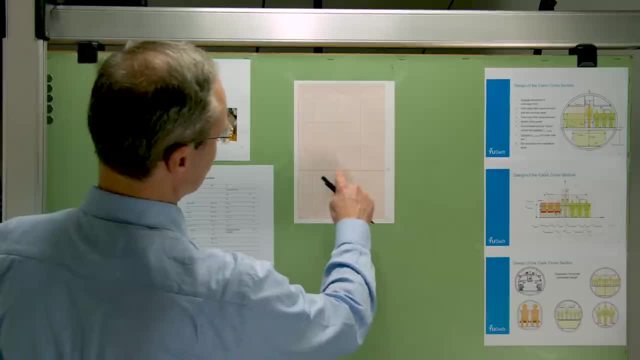 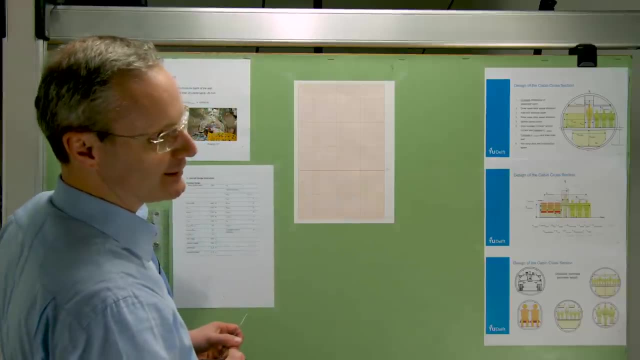 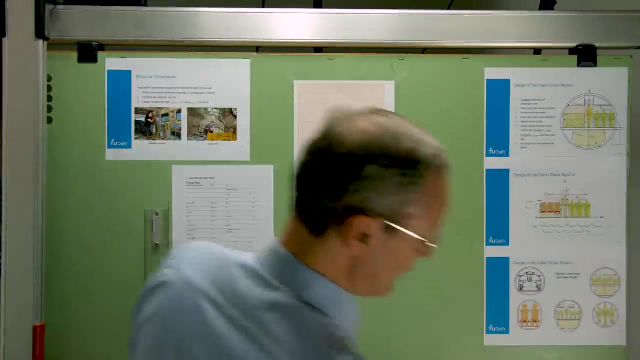 to be 38 mm above the floor line. The nice part of this graph paper is that this is indicated in mm, So 3.8 cm is a little bit less than 4 cm, And these blocks are 1 cm larger. 10. 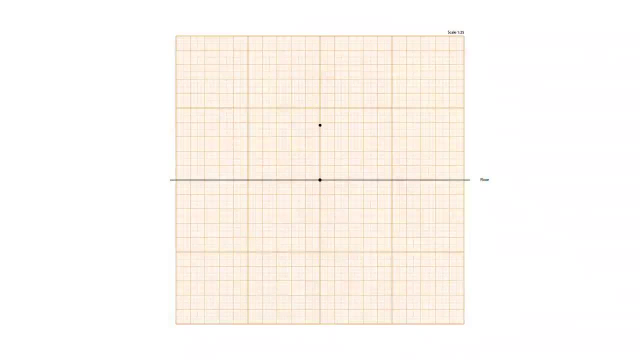 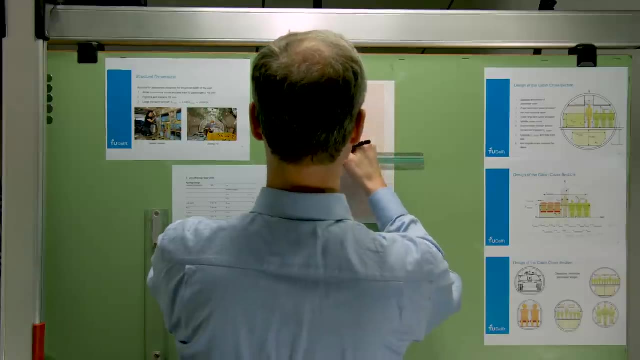 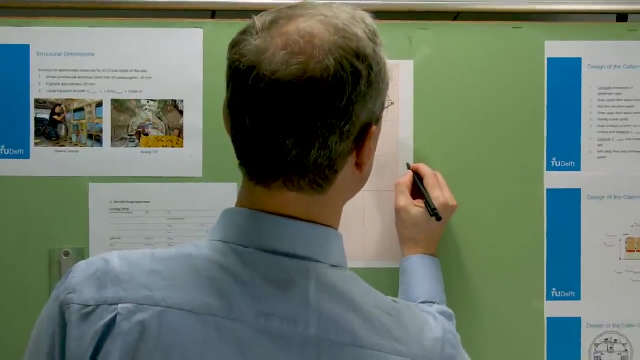 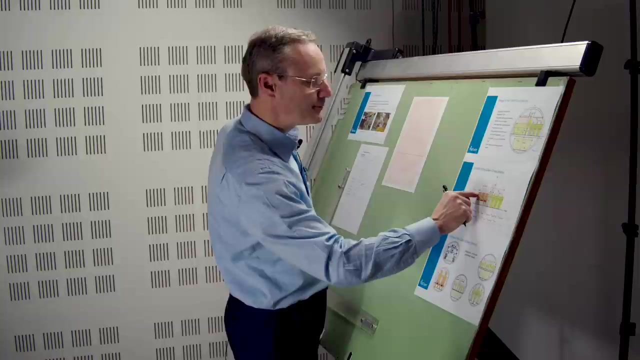 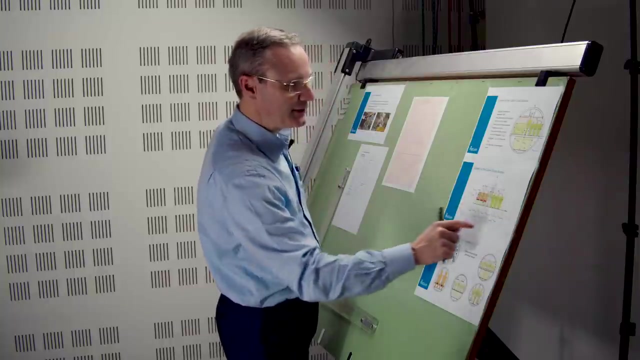 mm by 10 mm, So I can use this one Again. I'm just going to draw a parallel line for the. So this is the line for the shoulder height That's called H sub sh. Okay, now we have done this line. Then we need the width. here And there we need the 3.19 meters. So what? 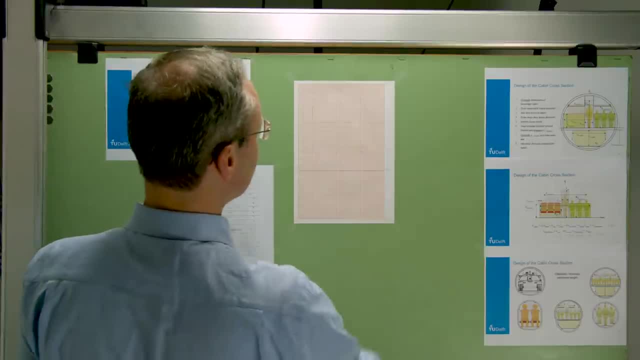 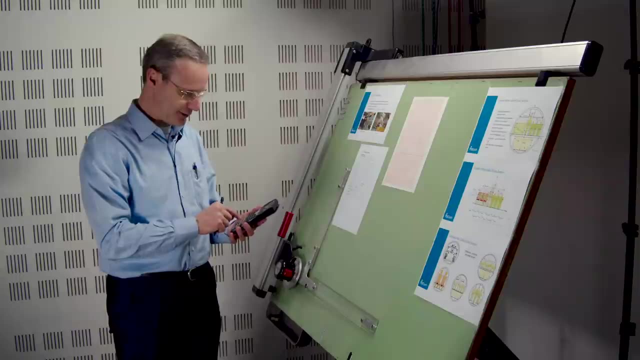 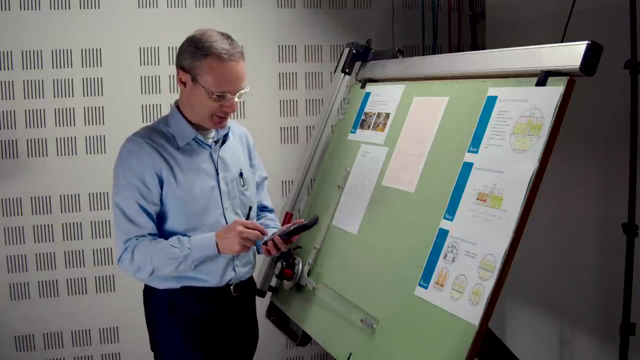 I'm now going to do is make a block, a rectangle on the floor, which is 3.19 meters wide, And then using the scale 1 to 25.. So 319 cm divided by 25 is 12.76 cm, So I need a space of roughly. 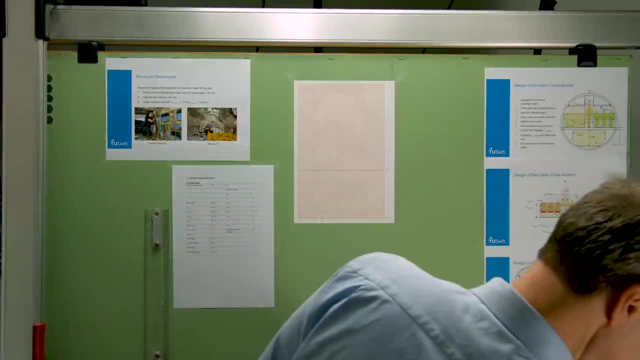 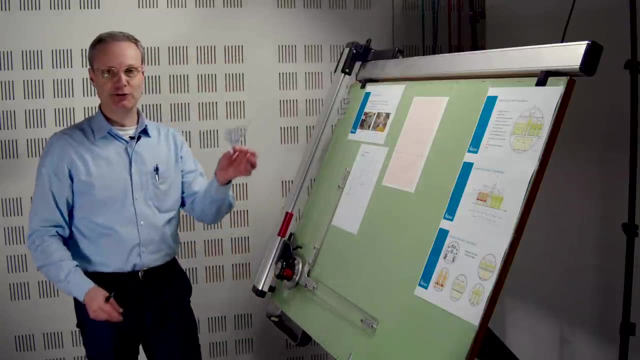 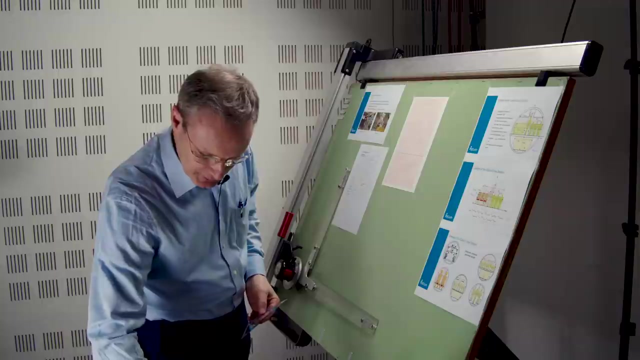 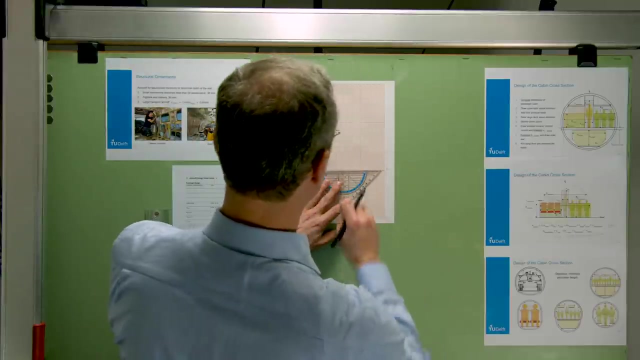 12.8 cm To make the drawing a bit more symmetric. you can make use of this device now because it has an even distribution from the middle. So what I need to do, I need to divide this by 2.. So 6.38 cm, so 64 mm, And I'm going to make this more or less in the middle of. 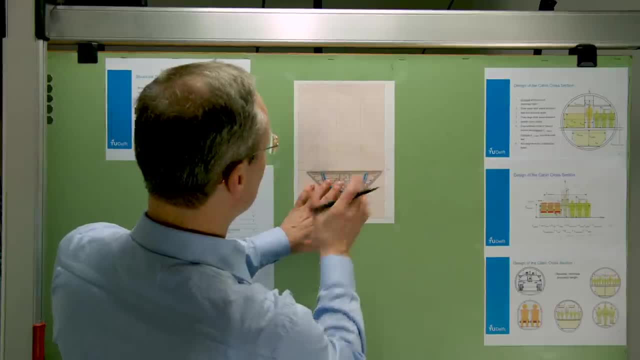 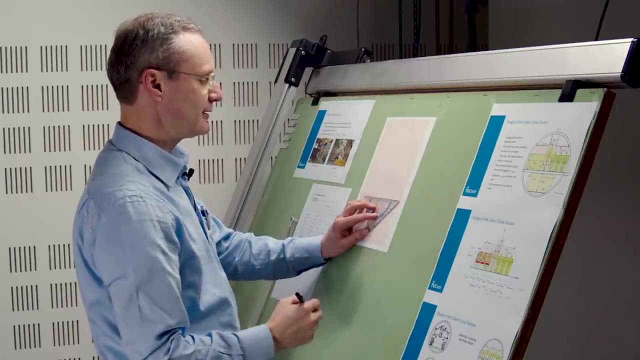 the picture, And it doesn't really matter whether it's really aligned or not, but more or less in the middle of the picture, And then I'm going to draw the line. So let's say, I'm going to use this point as my center line, and then I'm going to be 6.4 cm to this side, 6.3cm to this side, 6.34mm to this side, But later on I need〜you know 6.14 cm to this side or 6.12 cm to this, anotherCo b, But later on it will look better. So I'm 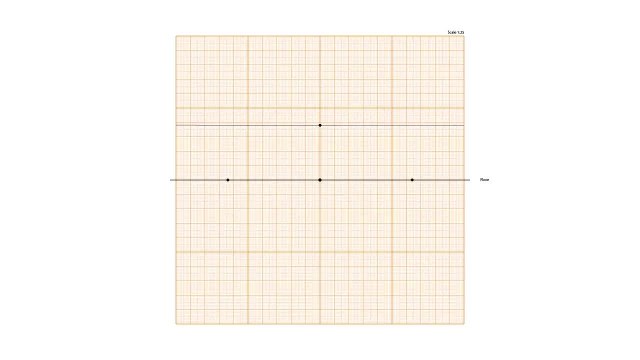 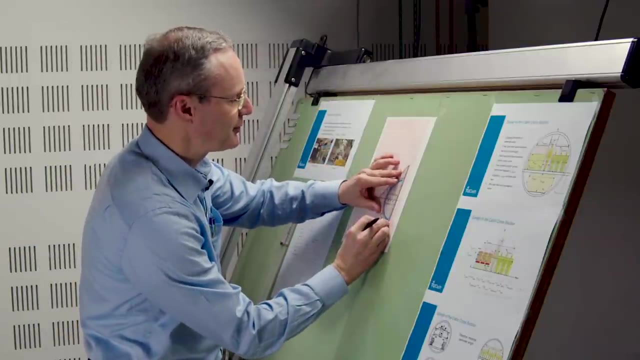 going to spend this time here, So obviously what I have done is divide this by two lines: The two and 6.4 centimeters to this side, and the nice part of this thing is that you can make perpendicular lines. so now we need to draw a perpendicular line over here. 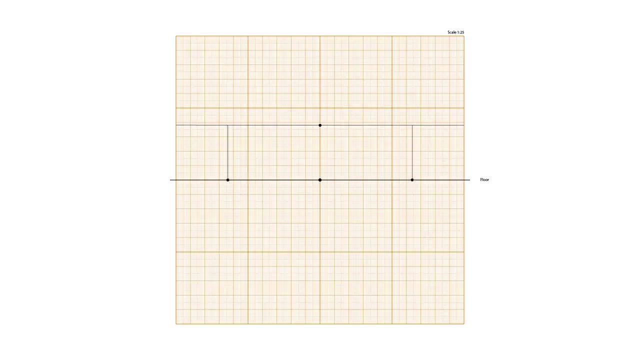 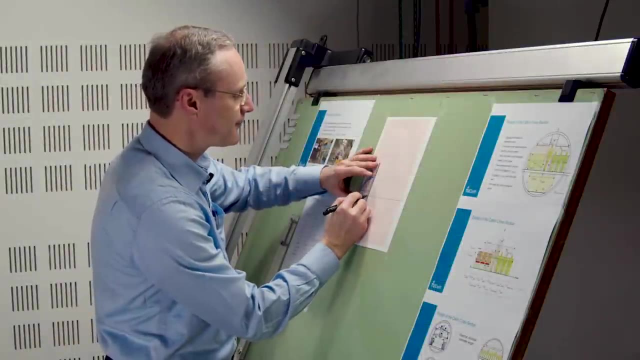 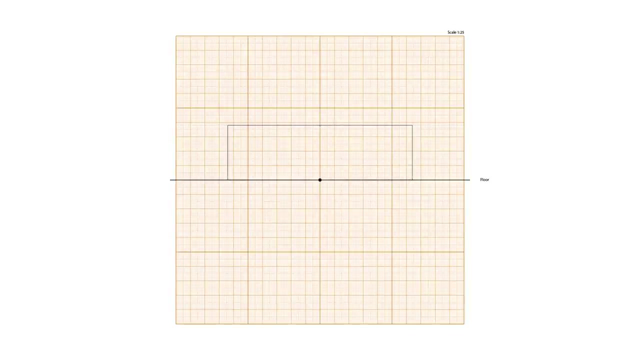 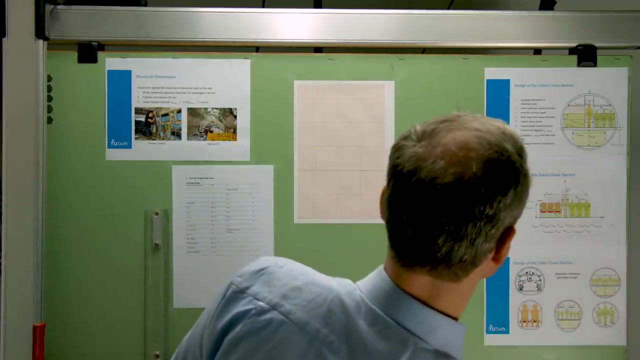 from the floor to the shoulder height, and we'll do the same over here. You can nicely line this up. and then we have the block for the shoulder height. Now we have just drawn this block. width of the cabin, shoulder height all inclusive. Now we 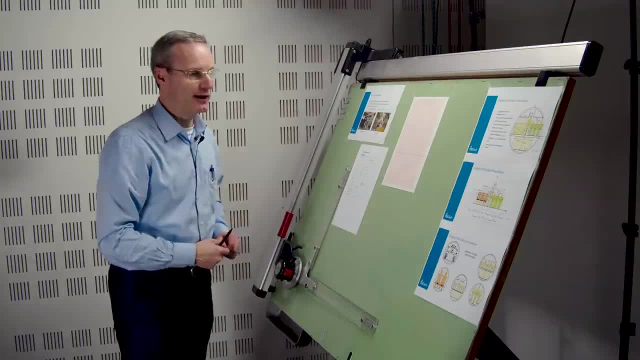 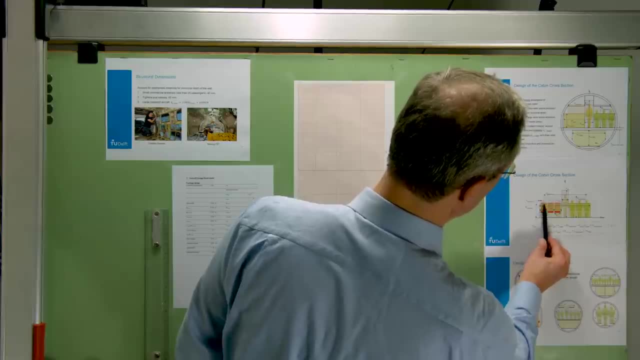 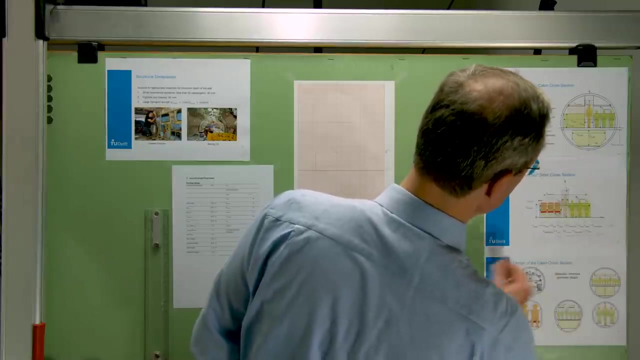 need to take the headroom, and the width of the headroom is centered around the seats. One edge lines up at the middle of the most headroom, The left-hand seat, and the other one lines up at the center of the most right-hand seat. So what we need to do from the edge of this block, we need to 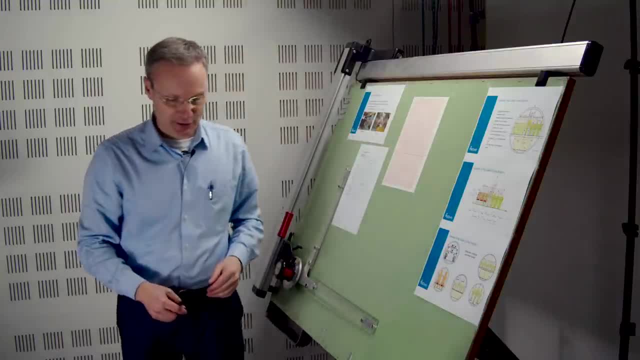 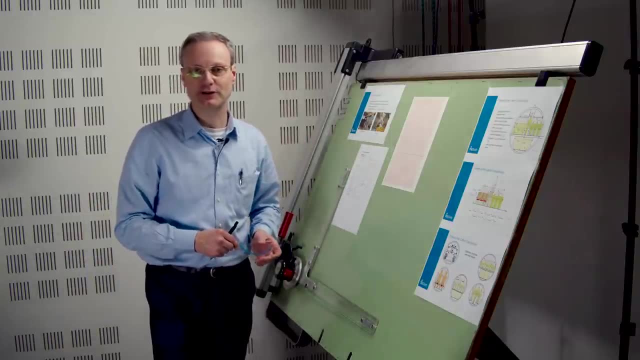 go inward on both sides. How do we do that? Well, it's the middle of the seat. the seat was 44 centimeters wide, so that's the half of the seat is 22 centimeters, but we must also take into account the fact that there is a 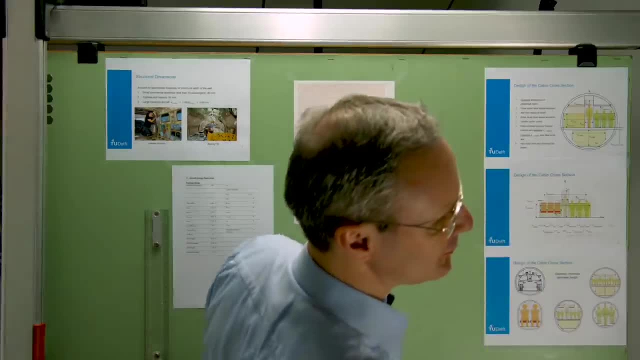 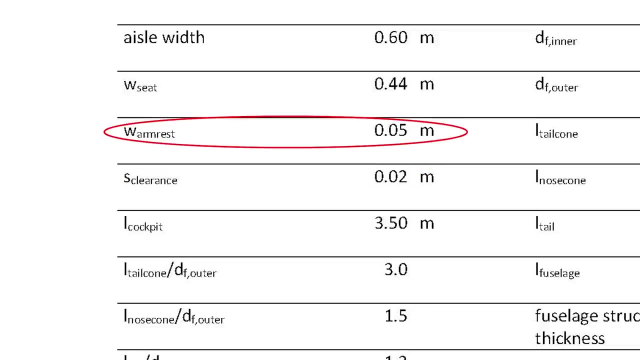 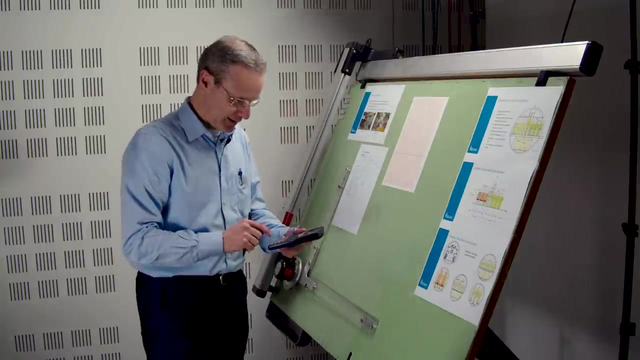 clearance and there is one armrest to be taken into account. The clearance from the table was 2 centimeters, the armrest 5 centimeters, so we go in 7 centimeters plus 22 centimeters from the edge. So we 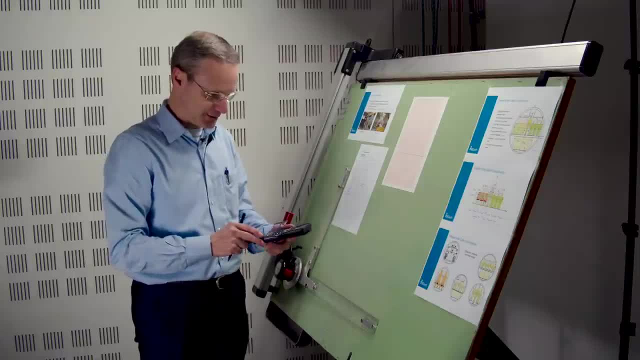 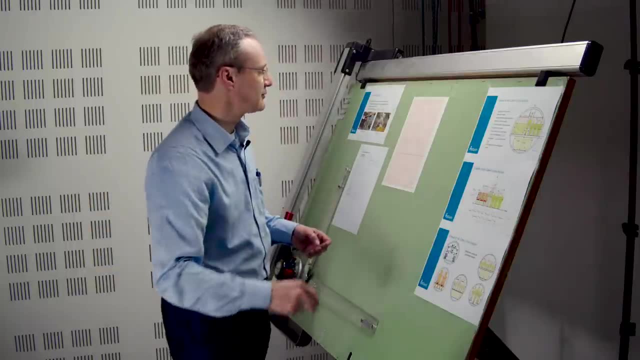 have 7 plus 22 centimeters is 29 centimeters divided by the scale 1 to 25 again. so it's roughly 1.2 centimeters, 12 millimeters. So we go in 12 millimeters a. 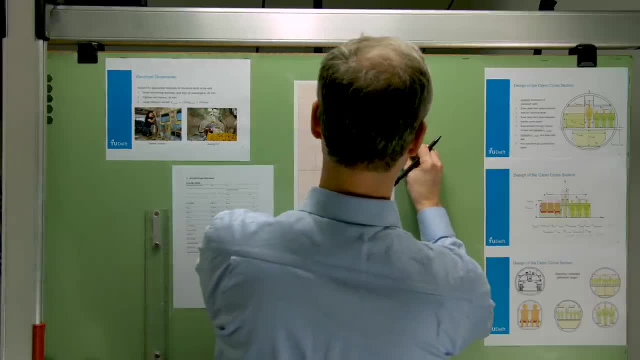 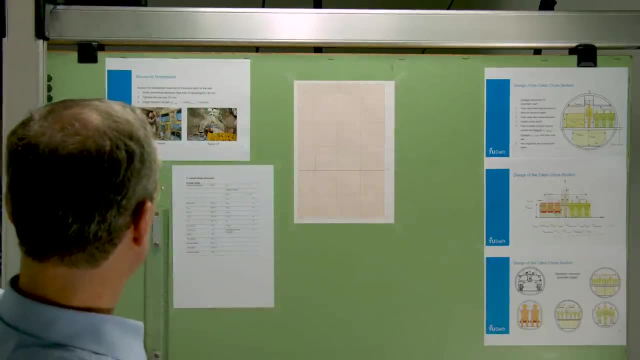 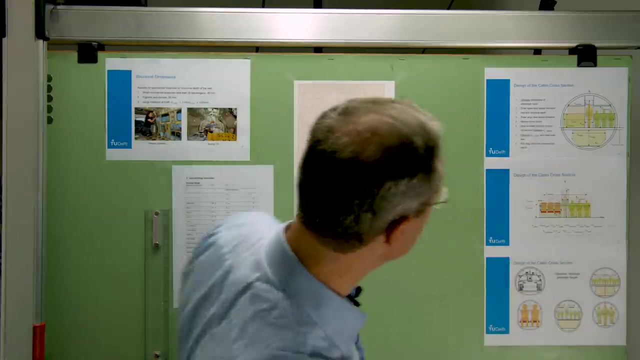 this side. This is from this side. of course we'll do the same from the other side, 12 millimeters from this side. And then we need to make this such that we also draw in the headroom height. so this height we have over here, that has been given as 1.5 meters, 1.5 meters. 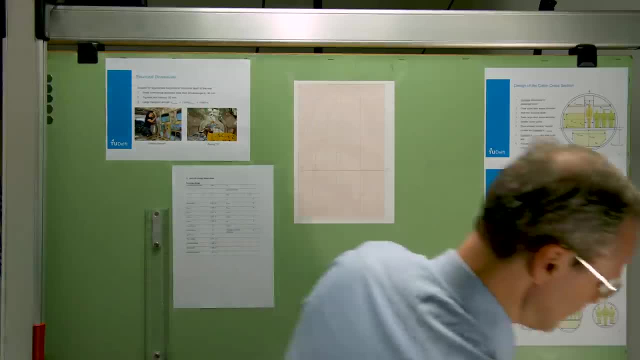 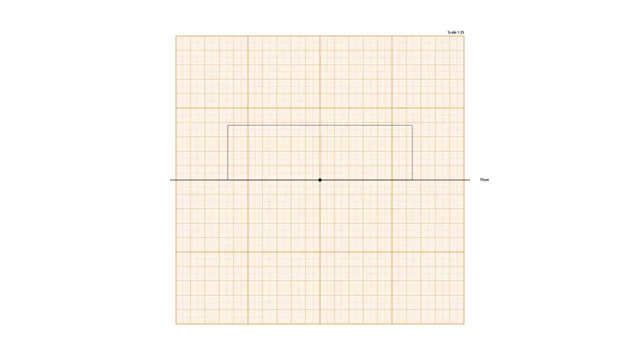 under the 50 centimeters divided by the 25 gives me 6 centimeters, 60 millimeters. So we need to go up from the floor at this point to a height of six centimeters. We'll do the same at the other side from the floor, nicely perpendicular. we go up to six centimeters And then we draw a. 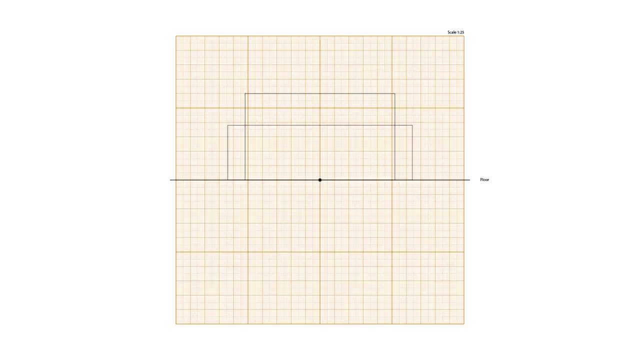 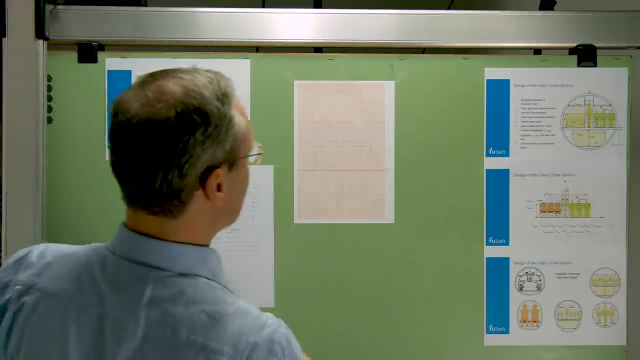 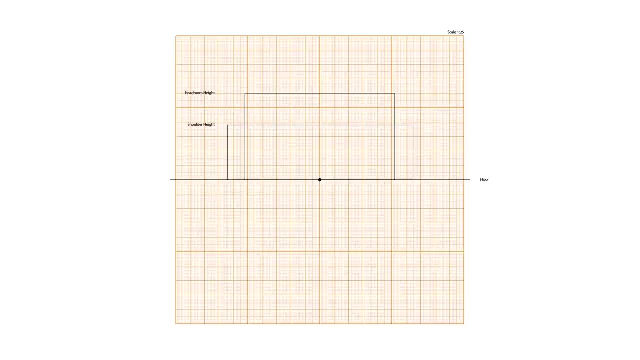 horizontal line again, And you can do that with the ruler or with this protector, And then we have the headroom room height. so let's make it here. here we have the shoulder height and here we have the head room height. if you like, you can draw in all the seats, but that's. 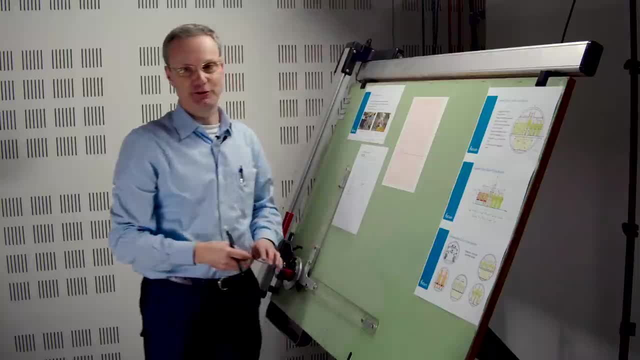 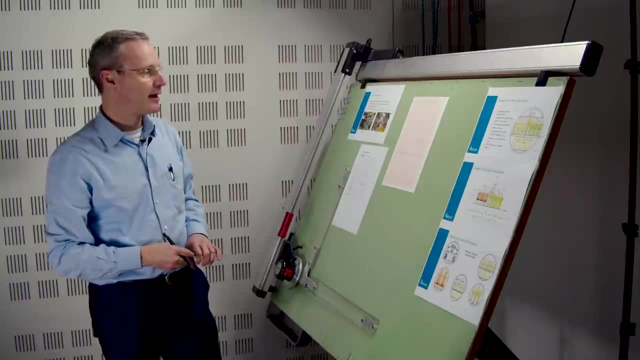 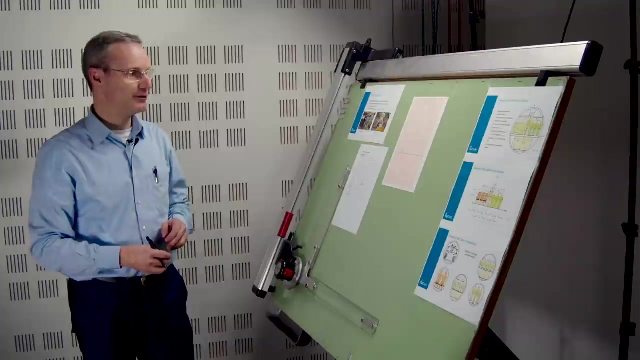 not required for finding the dimensions of the fuselage, but if you have some time left you can nicely draw the seats and armrest and all this kind of thing. but that's not really required and the next thing we need to do is to figure out where the aisle is, and the aisle is not in the center of the fuselage. we can. 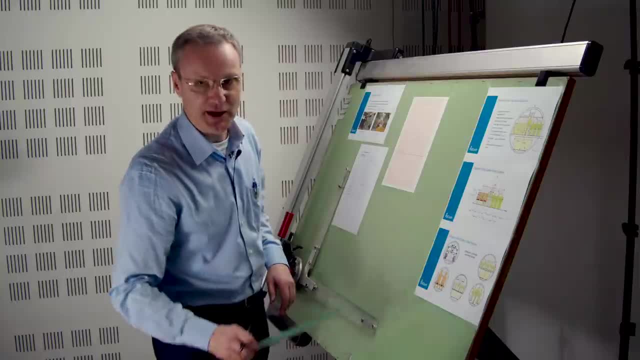 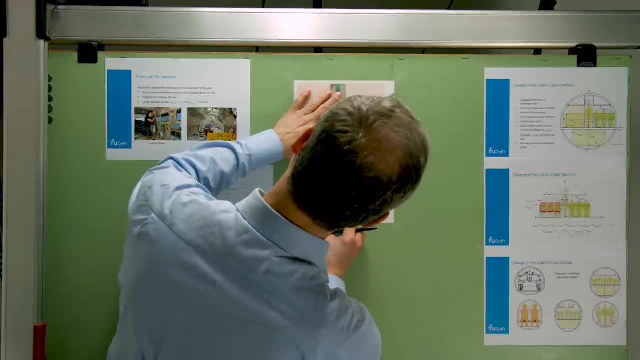 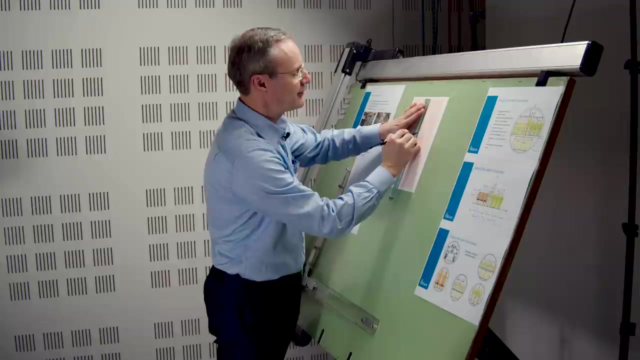 draw the center line of the fuselage in the meanwhile, because we have chosen a center line point, because we chose this point, so in principle we can already now draw the center line of the fuselage, at least the vertical center line, that will do. we have a dash dot line which is the center line of the fuselage. 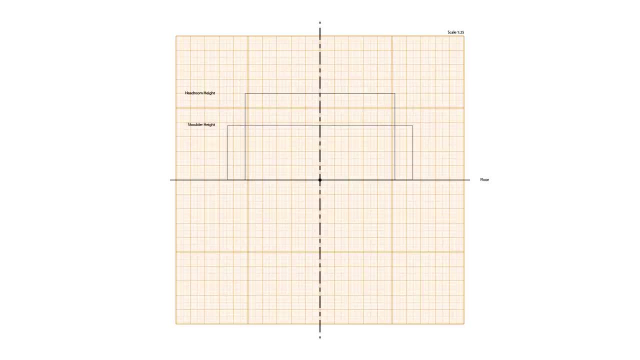 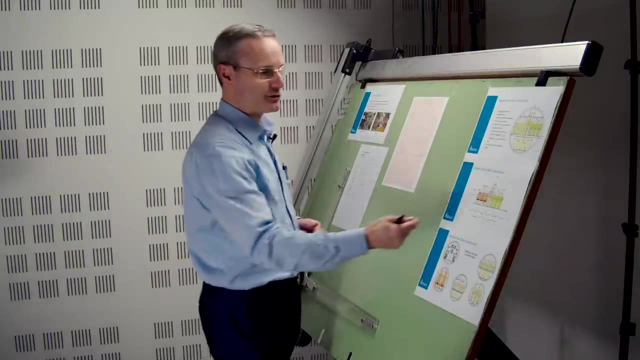 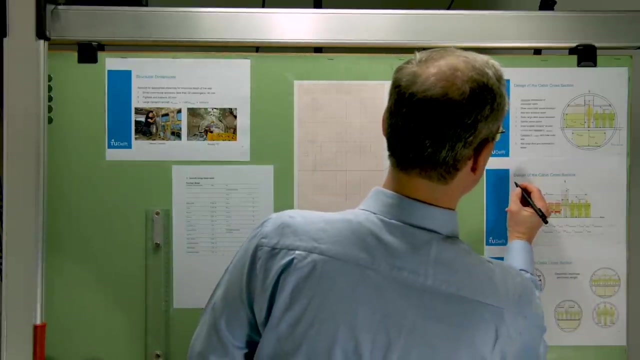 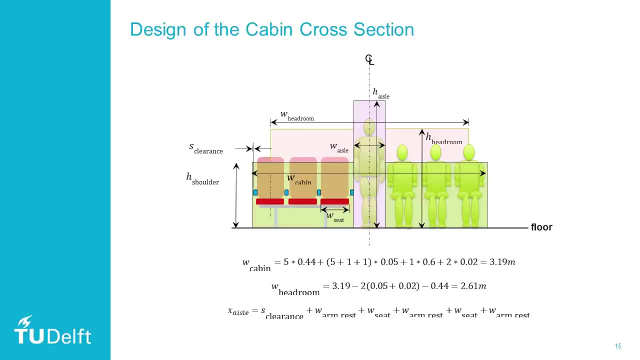 so here we have the center line of the fuselage. now we need to figure out where the aisle is, and that requires some calculation. again, let's do it from from the right hand side counting. we'll start here, at the far edge. we have a clearance. we have two centimeter clearance. we have, in this case, one armrest for this seat. 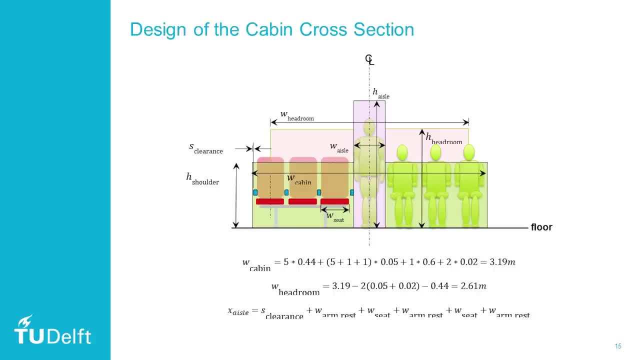 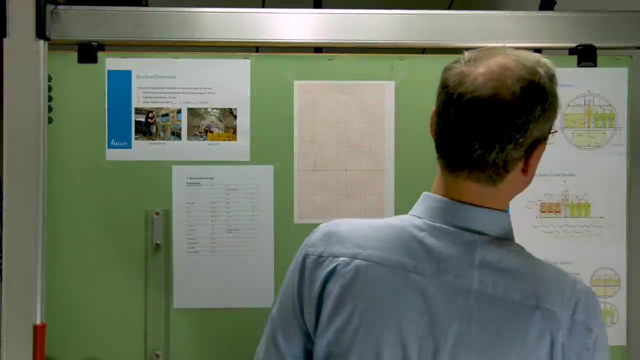 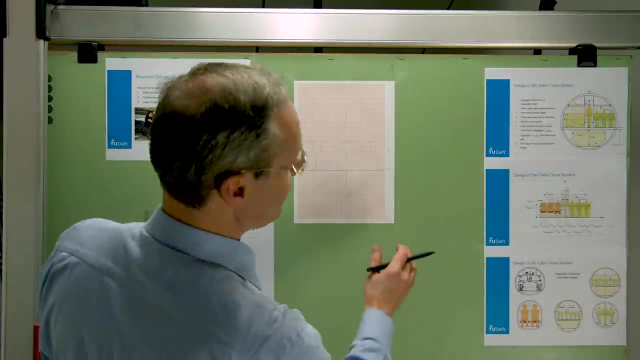 so that's five centimeters. we have one seat, 44 centimeters, plus another armrest, 0.05 plus another seat plus another armrest, and then I have the edge of the aisle here, assuming that I have two seats on the right hand side and then the remaining three on the 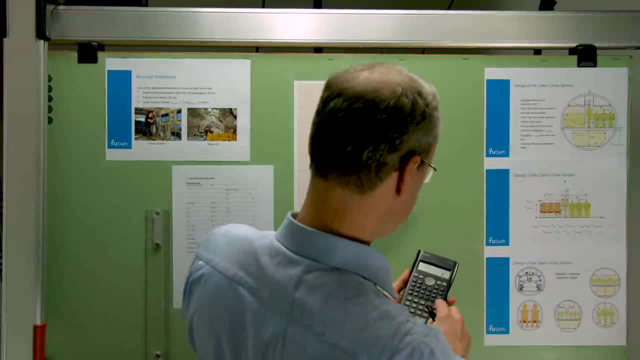 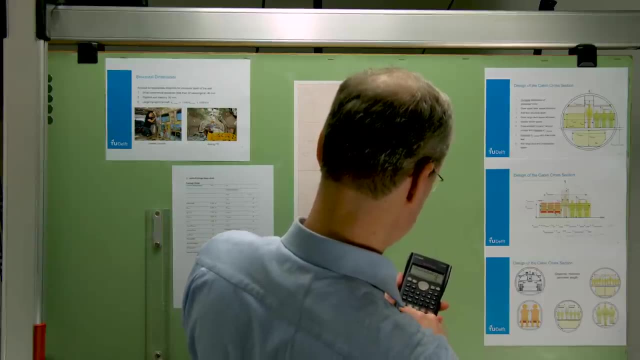 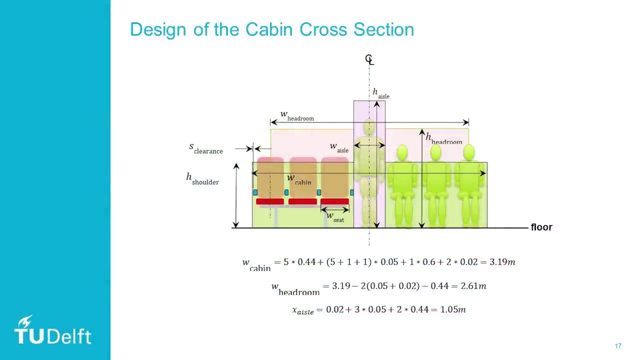 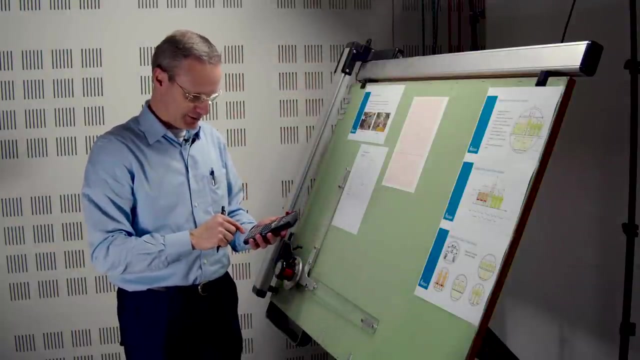 other side. so let's add that up, we have 0.02 plus 0.05, plus 0.05 plus 0.44, plus another armrest, plus another seat, plus another armrest, that is 1.05 meters. 105 centimeters divided by 25 again, that's 4.2 centimeters 42. 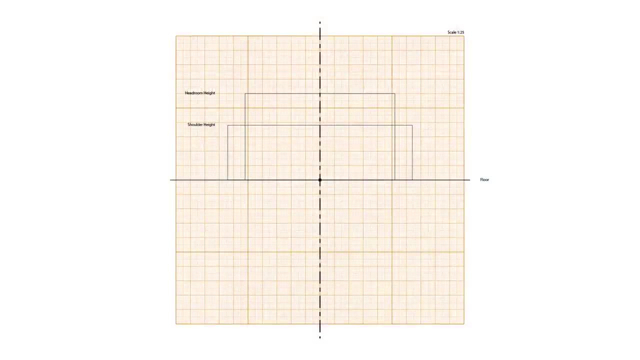 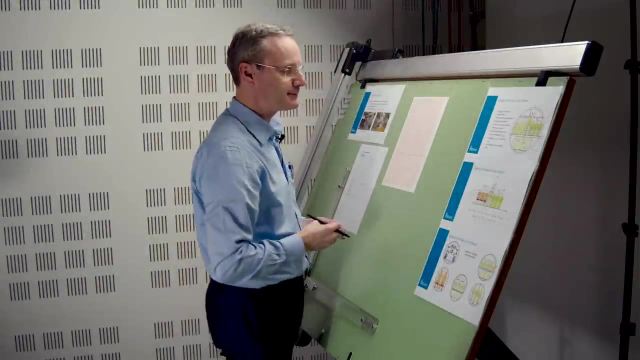 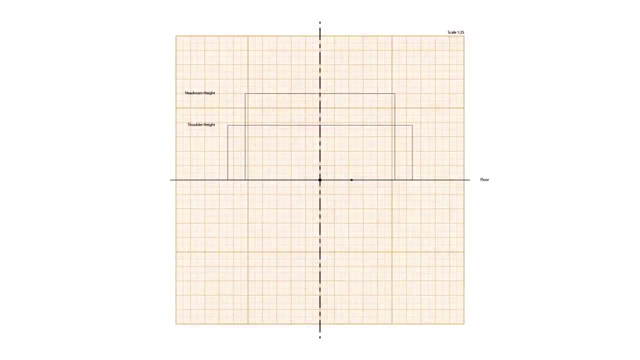 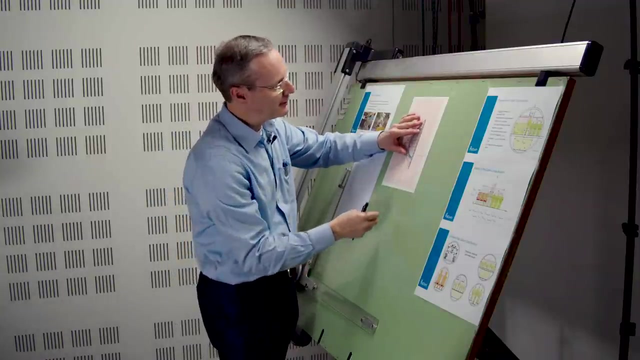 millimeters, so my aisle is going to start 42 millimeters from this edge. so I'm going to start 42 millimeters from this edge, I'm going to be over here and can draw a vertical line over here. and now you probably see that you run into the limitations of this device, so you need 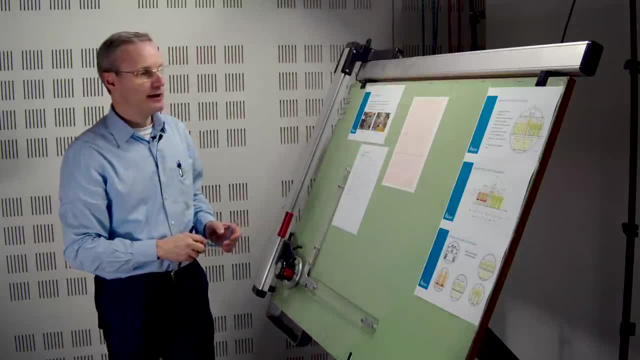 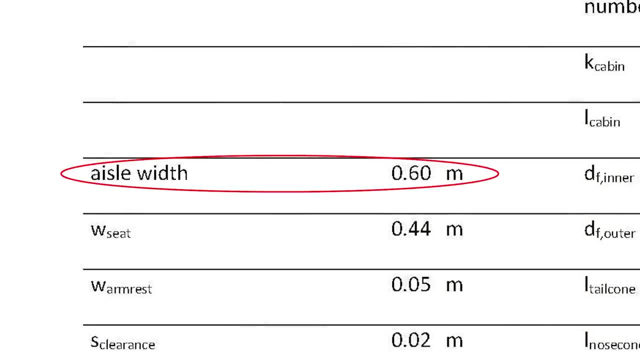 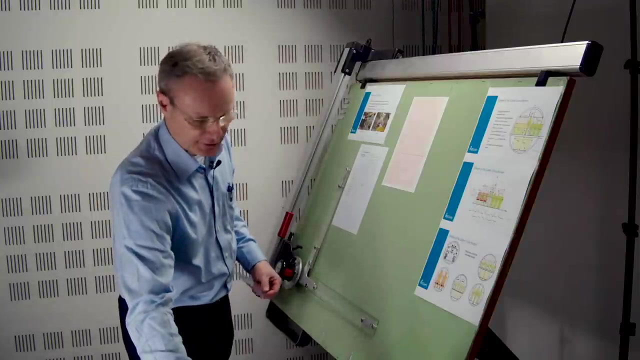 to move it up if you want to go further, but I'll talk about that in a second. and we need to take into account the width of the aisle has been given as sixty centimeters. centimeters divided by 25 is 2.4 centimeters, 24 millimeters. so from this point on, let's. 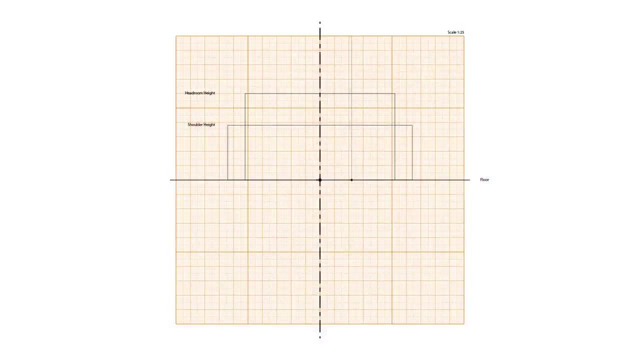 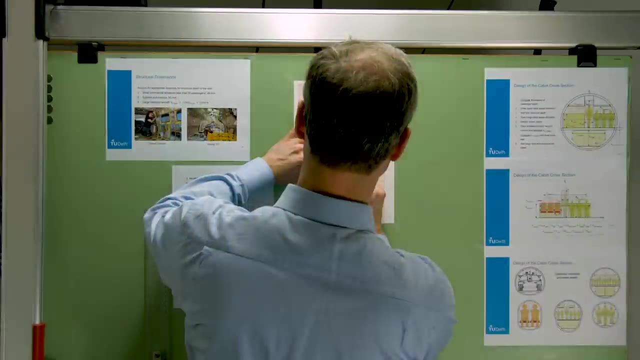 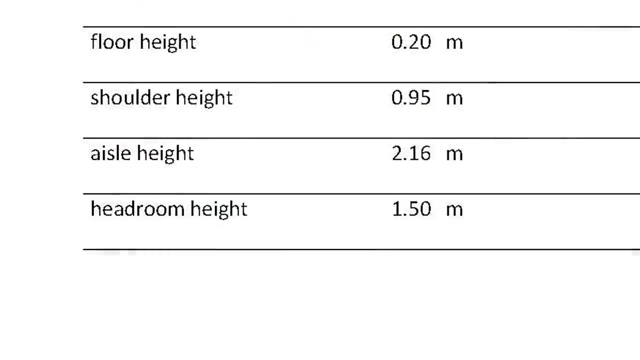 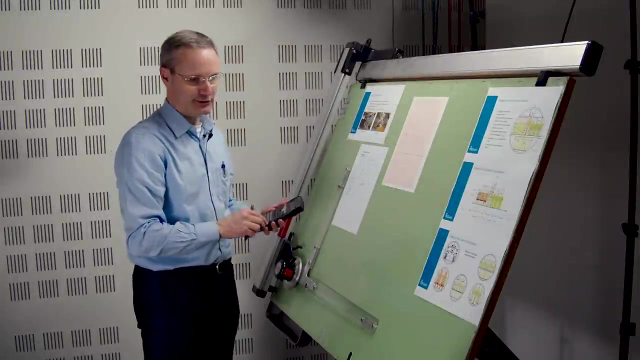 start here, at the bottom: 24 millimeters, 24 millimeters over here make a perpendicular line, and now we need to figure out what is the height of the aisle. that has been given as 2.16 meters. let's do the calculation again: 216 centimeters divided by 25, 8.64,, 8.64,. 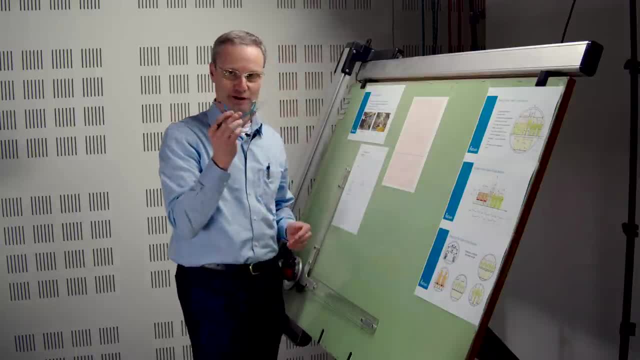 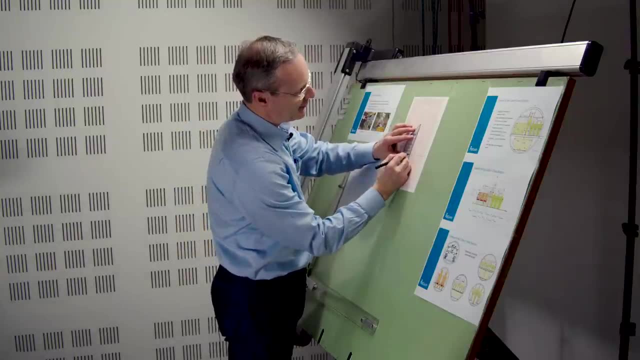 okay, we need 8.64,. you will see that this device only runs to 7 centimeters and not to 8, so you need to move it up. let's move it up to starting at 2, and then we have 8,. 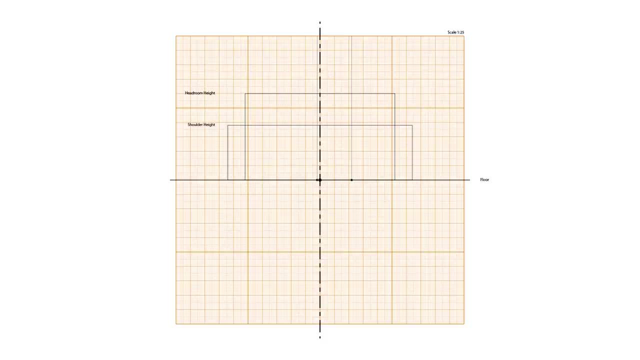 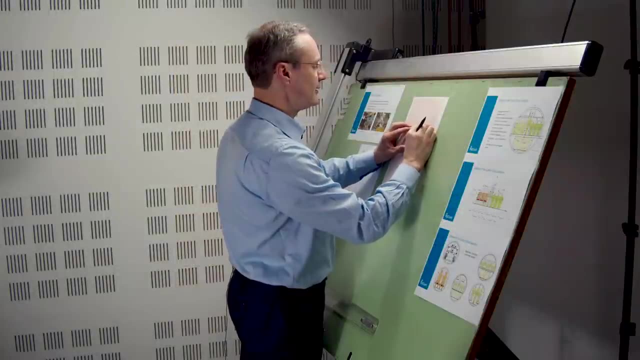 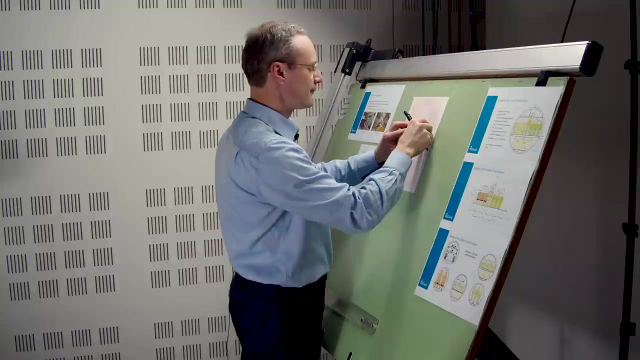 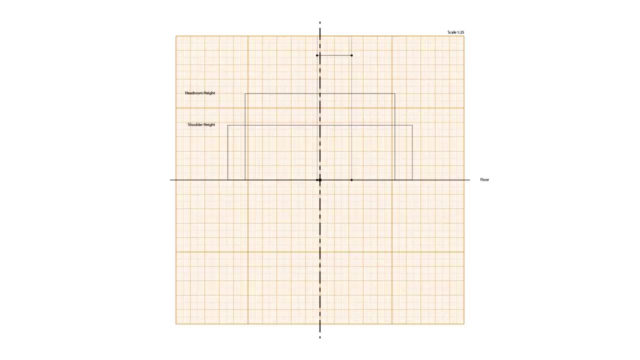 8.64 is roughly here, So this is going to be the height of my aisle. make use of the nice perpendicular lines on the graph paper to make nice perpendicular lines in your drawing. so here we're going to have the top of the aisle. we can now extend the sides of the aisle and then we can nicely. 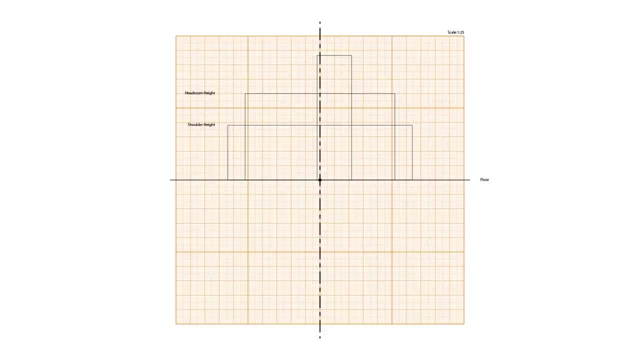 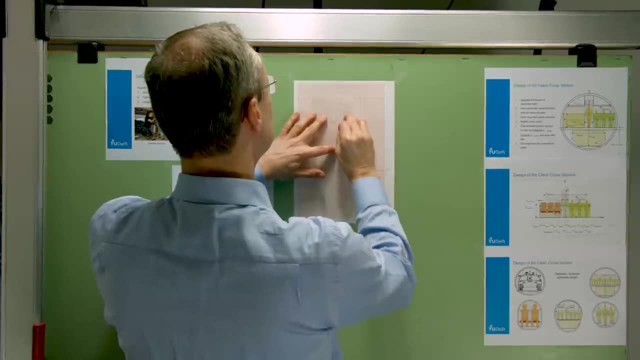 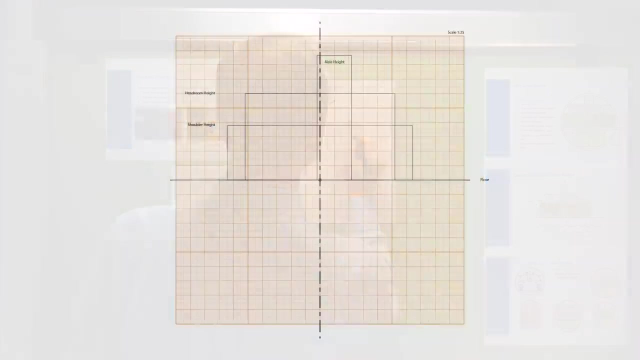 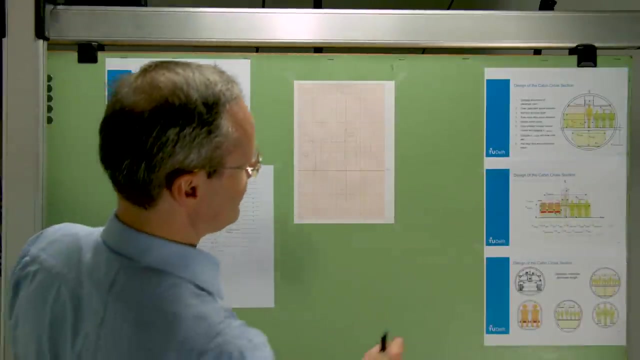 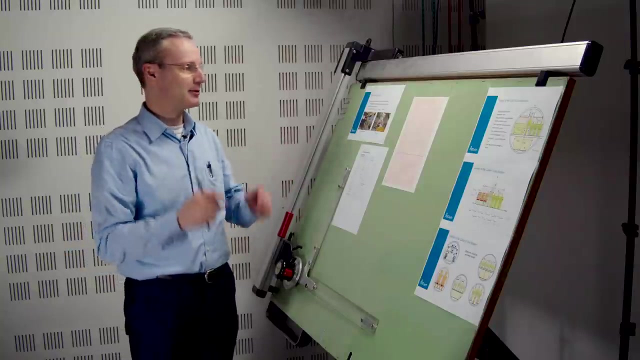 complete the aisle, use the eraser again to get rid of the lines which are not necessary anymore. And here we have the eye height and also the width, of course. So now we have all the elements in this diagram And that means now we can try to figure out what is the smallest diameter we can. 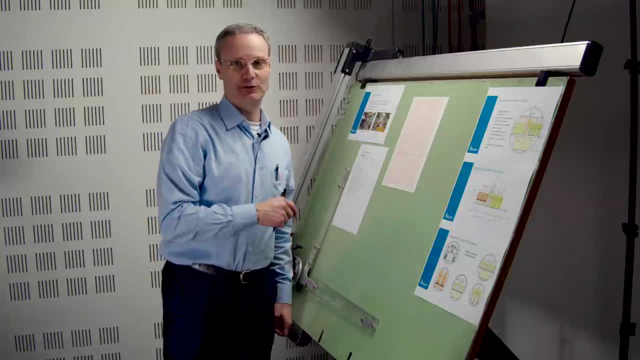 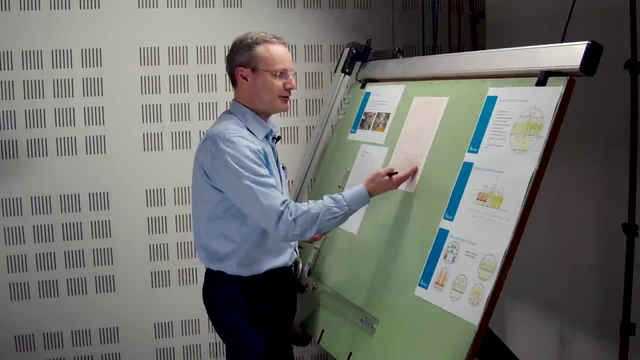 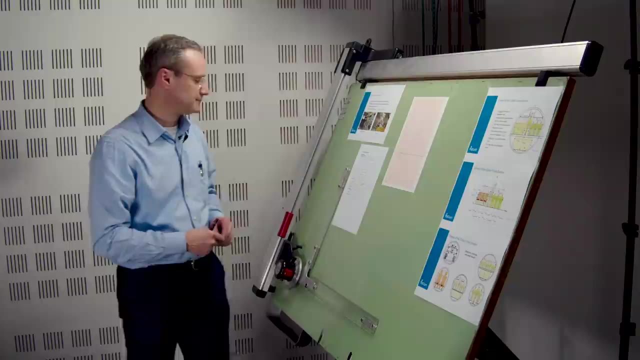 draw around that In this case there is no cargo in the assignment. If there would have been a cargo requirement, we would need to take into account the space here, And if you want to do that, you first need to draw in the structural thickness of the floor. Well, has there been something given about? 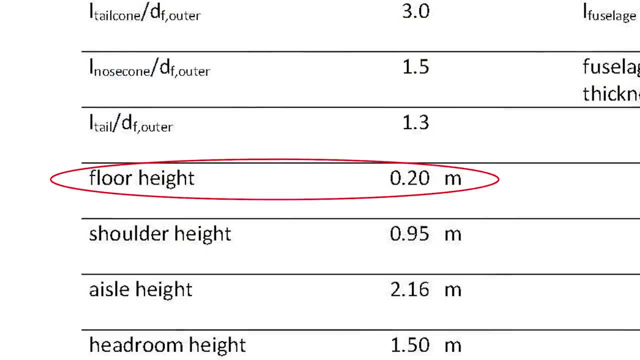 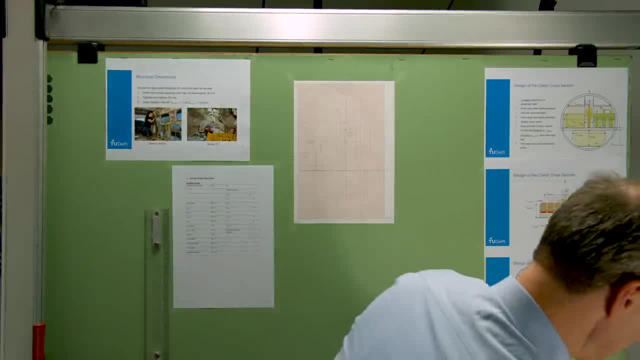 the structural thickness of the floor. Well, there is no cargo in the assignment, So now we have. Yes, the floor height has been given as 20 centimeters, 0.2 meters. So 20 centimeters divided by 25 would have been 0.8 centimeters or 8 millimeters. 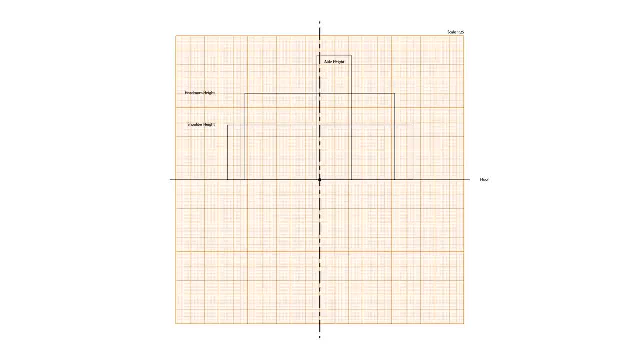 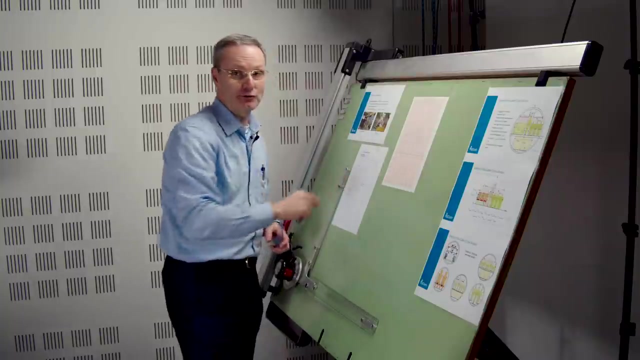 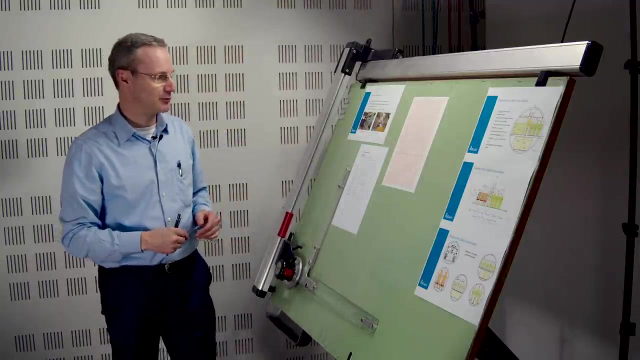 So you would need to draw the floor height in there. This is the structural thickness we need for the floor- And then you would need to draw a cargo container here, or suitcases or whatever. In this case that was not required, But you would need to do that if that would be required. 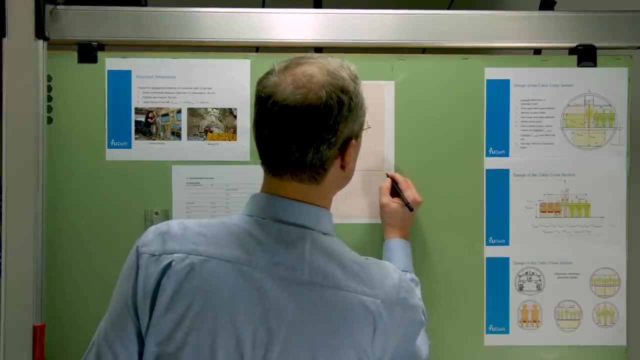 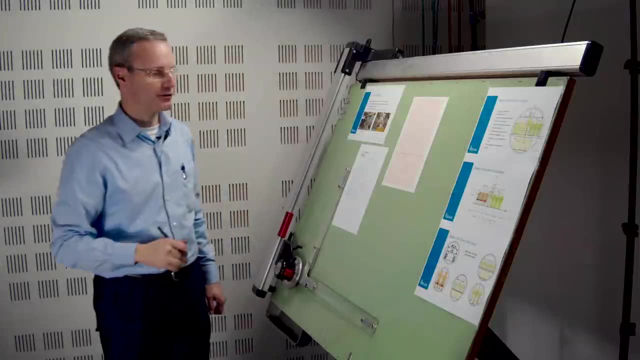 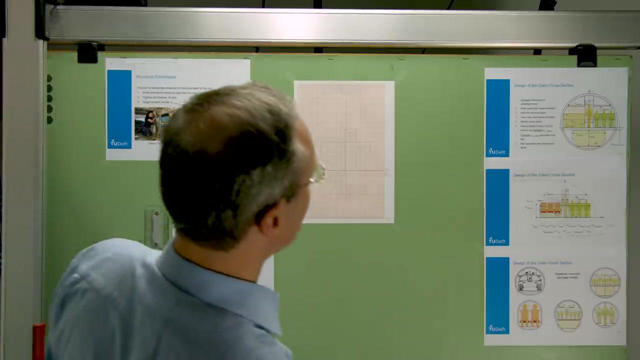 So here we have the floor thickness. Let's write it here: floor The floor thickness. but we don't need that. So now we can move on without any problem. The next step, because now we're more or less really quite a bit way on our way in our plan. 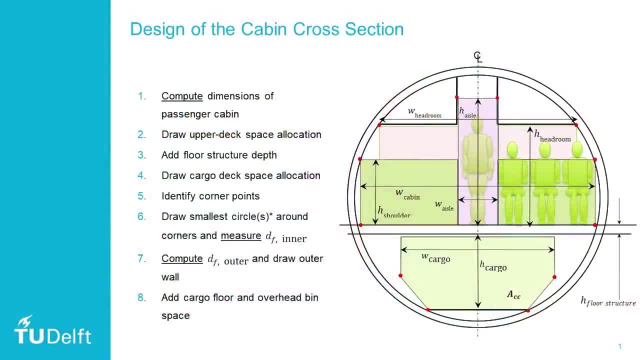 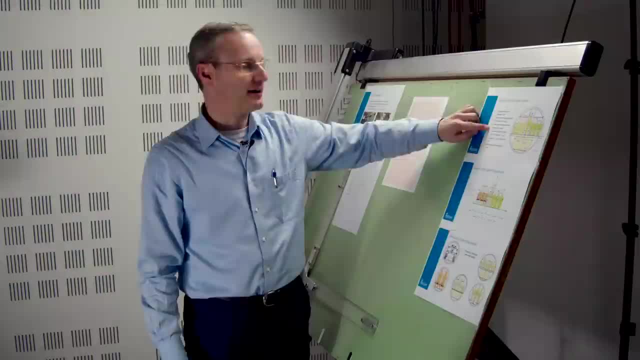 We have the dimensions. We have the upper deck space allocation, We have the floor structural depth. We have, in this case, no cargo, And that means we're now at step five. We need to identify the corner points. We have corner points. 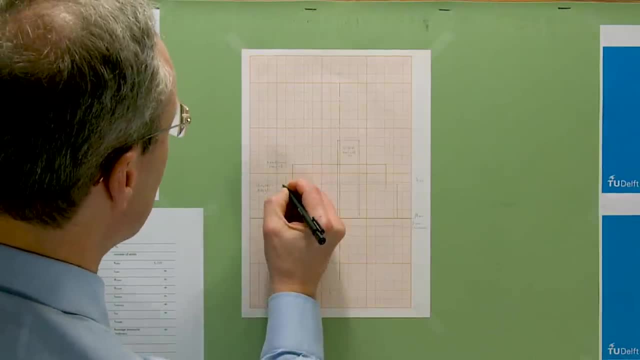 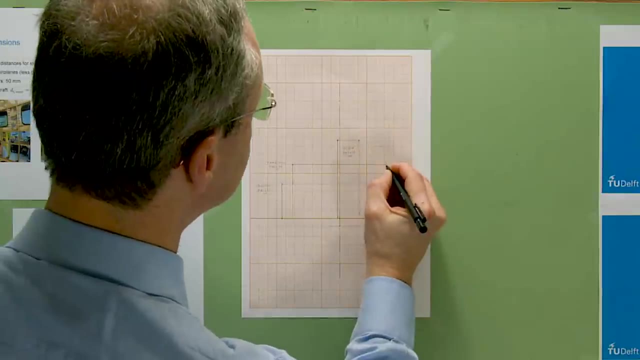 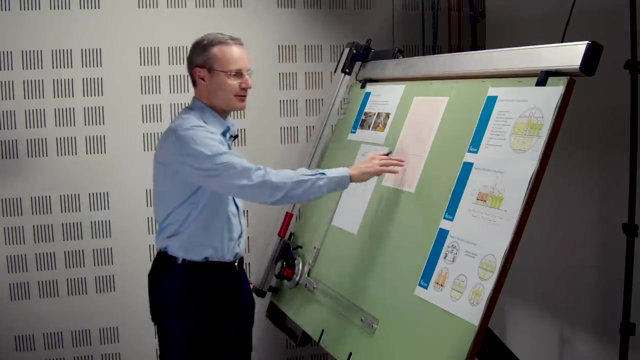 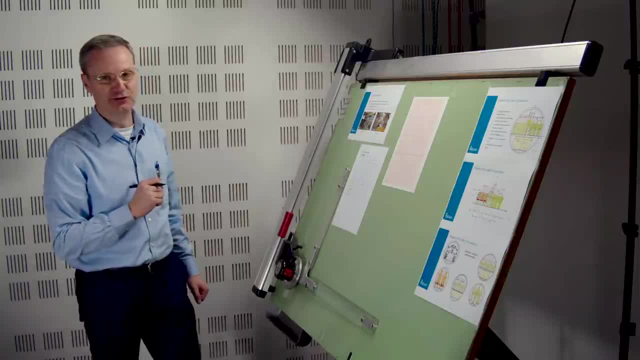 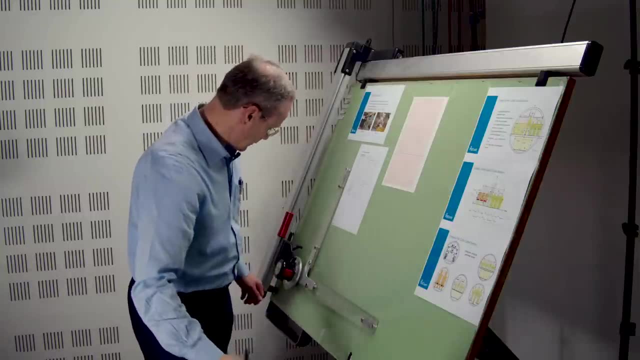 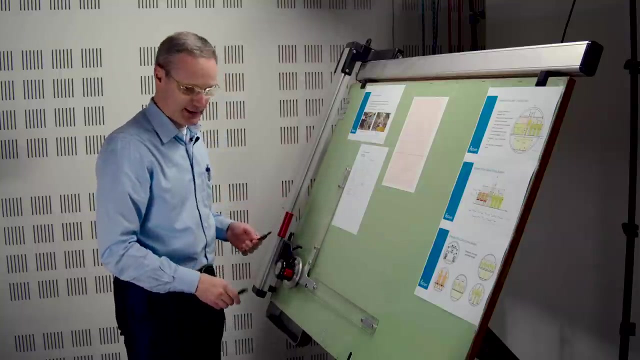 And now we need to find the smallest circle that you can draw around this point. You can do that with a lot of trial and error. Use this, the compass, the geometric compass, and try to figure it out. How do you do that? 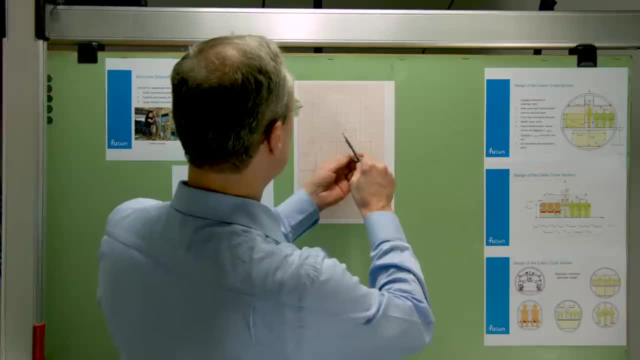 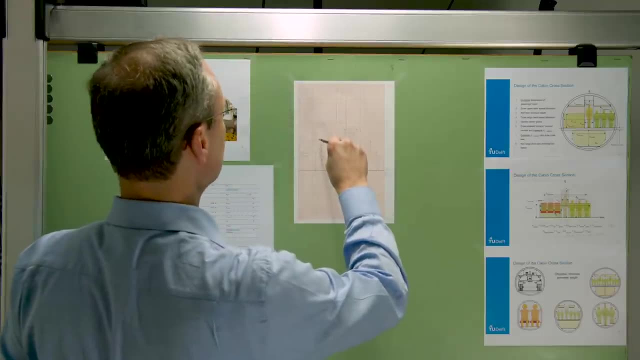 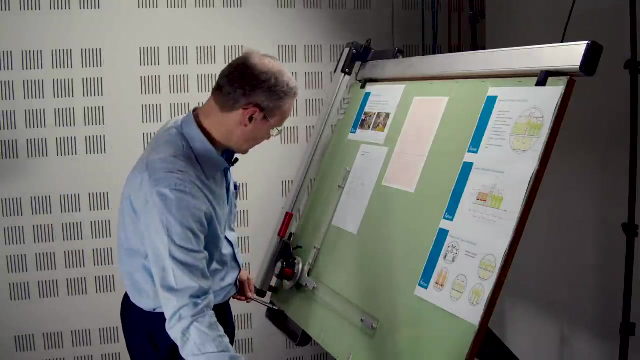 Well, in principle, you put the sharp point somewhere on the center line. That's why we need the center line in the drawing And try to find something which goes around it. But there's a smarter way to do that, And the smarter way works as follows: 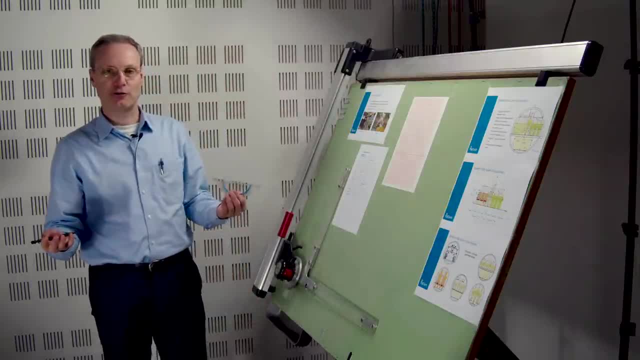 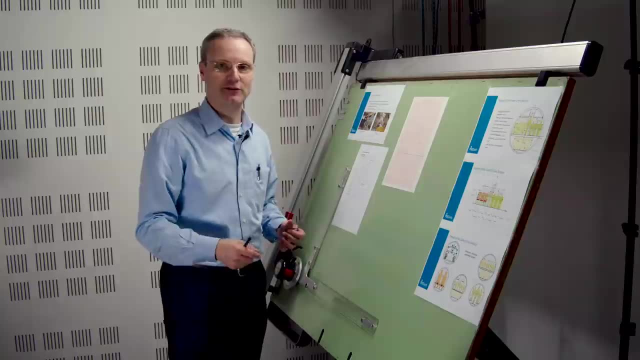 The first thing you need to do is to make an estimate of the corner points you think will be limiting. It's not a problem. if your first choice is incorrect, You can always correct it. That's why I use light pencil strokes. But let's suppose we assume that this point 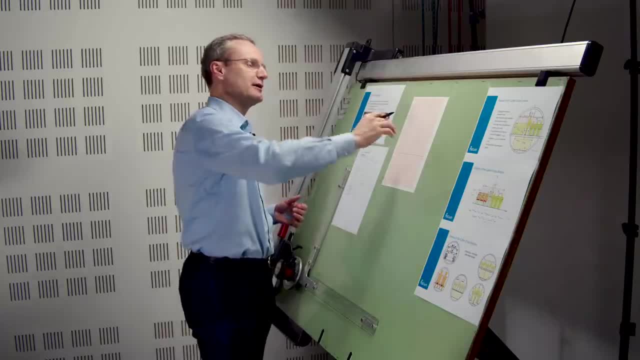 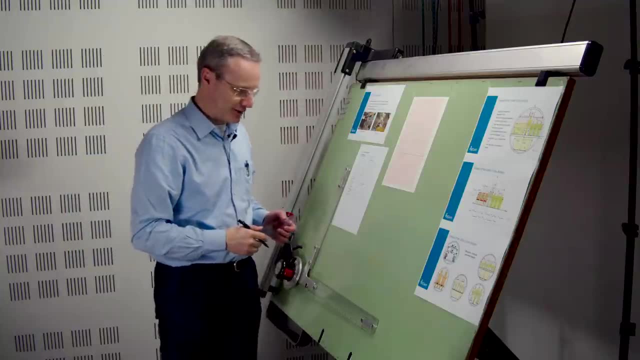 and this point is going to be limiting, That the circle has to touch these points, and that's going to be limiting. How would you then find the nearest circle? Well, effectively, what you need to do, you need to find a circle which has this point. 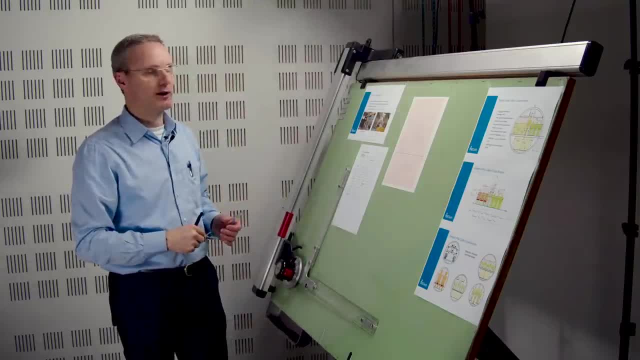 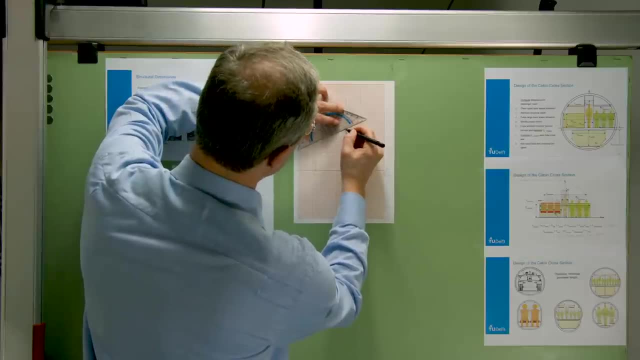 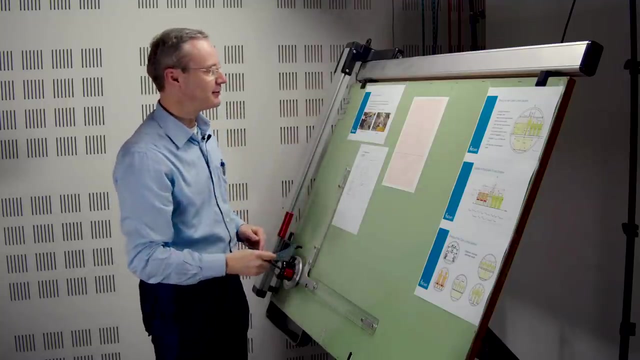 and this point. But that again requires some trial and error. But the fastest solution is as follows: You draw a straight line between these two points, Straight line between these two points. Then you reverse this triangle And then you're going to find the middle of that line. 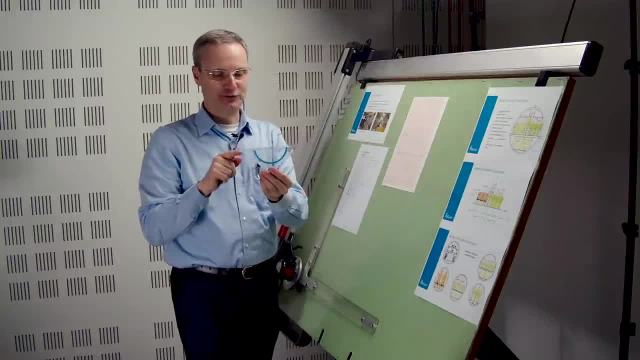 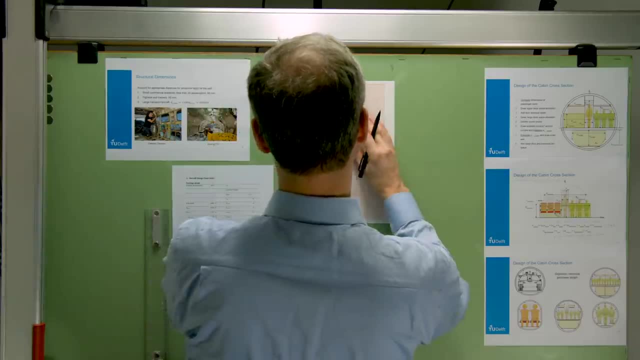 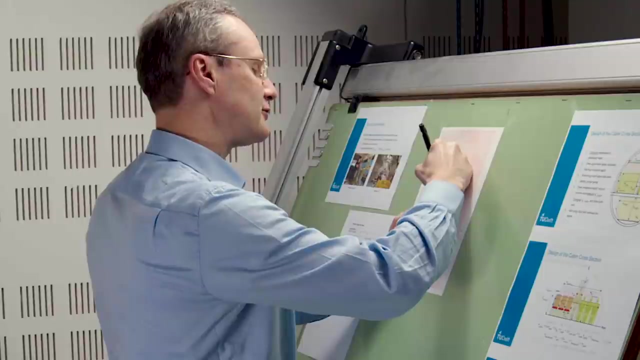 And then the nice part of this protector is that it is equally divided: Seven centimeters on this side, seven centimeters on this side, So it's easy to find the center, And that's going to be roughly. here I'm going to indicate the center of that line. 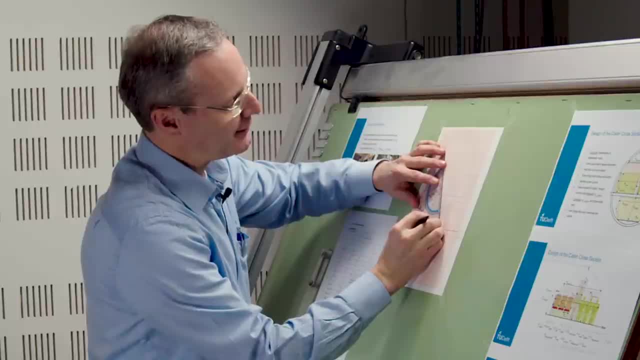 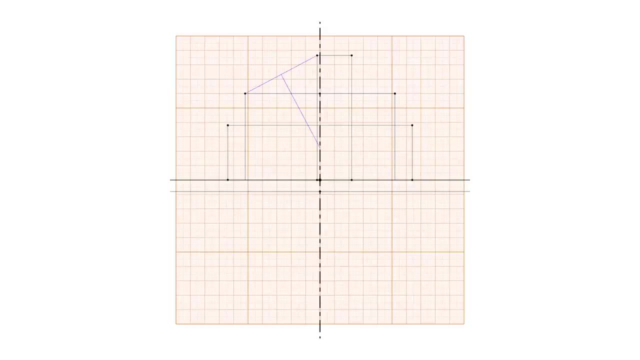 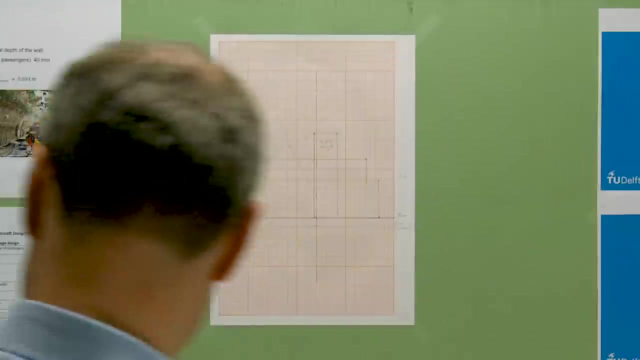 And from that point I'm going to draw a perpendicular line, again with the help of this device, Until I touch the center line of the fuselage, And then I find this point over here, And that will be the center of the circle. 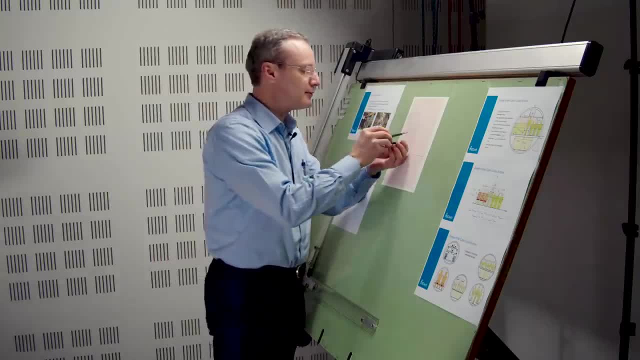 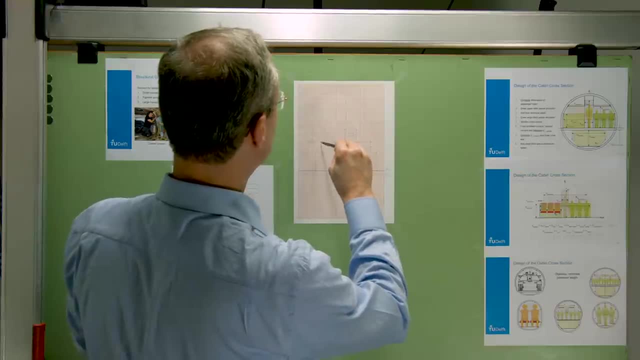 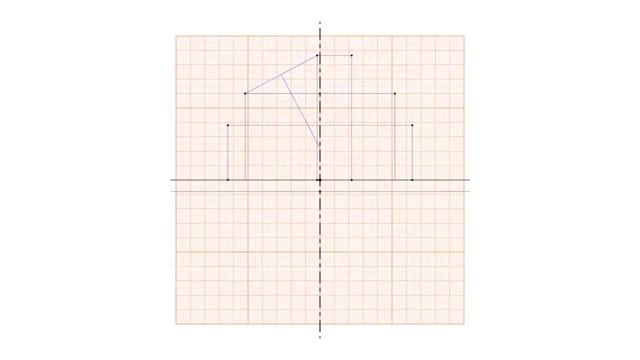 that will touch both points. I'll put the sharp point over here, I'll measure it such that I have one point and I will see that automatically I have this point as well, And then I draw my circle, At least the first estimate of my circle. 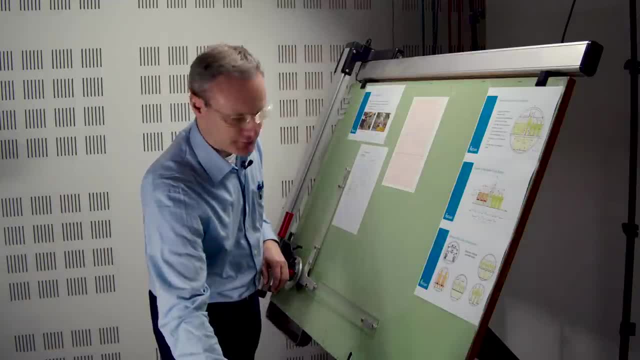 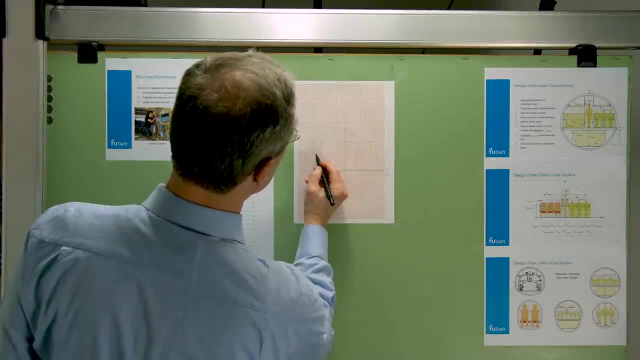 And what you see now? that this is not the correct circle, Because we will see that this point is okay. This point is okay. This point is not okay. That falls within the circle. This point is also not okay. It does not fall within the circle. 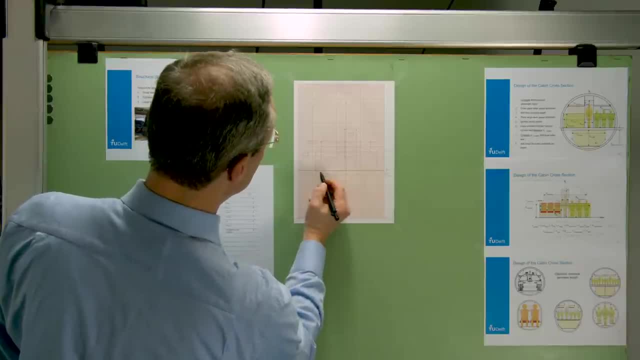 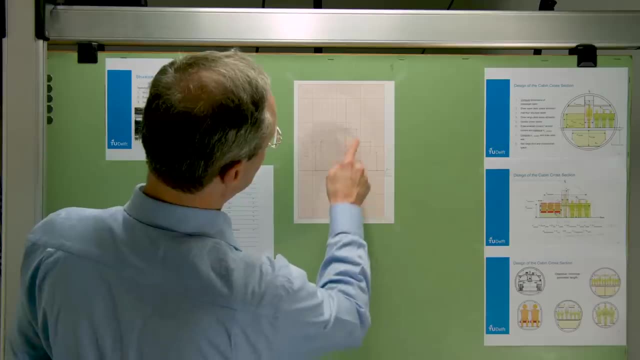 This one is okay, This one is almost okay, And this one and these ones are okay. This is not the correct circle, So we need to do another attempt. So my next attempt is going to be to look at these two points, So that might be the critical point. 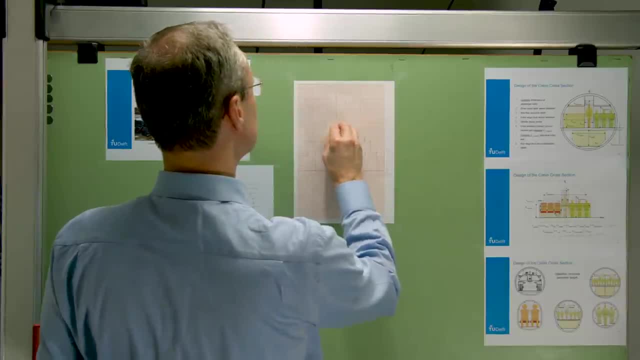 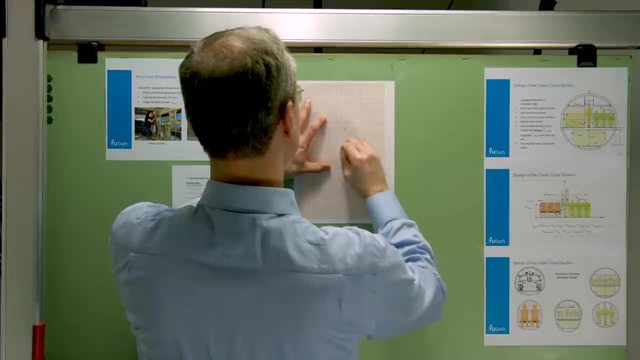 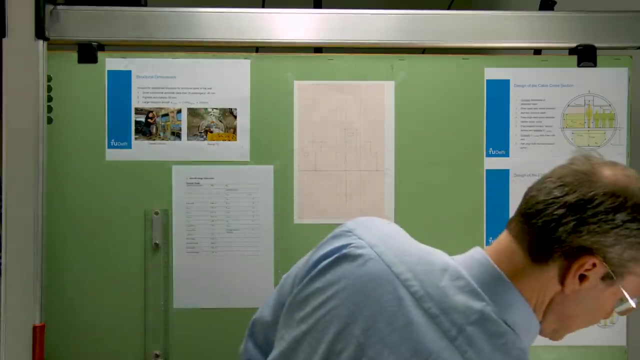 So here you see the benefit again of using light pencil strokes, Because now you can remove the incorrect circle, You can also remove the additional line. Let's do it like this And again use the same trick. My guess is that this one and this one might be limiting. 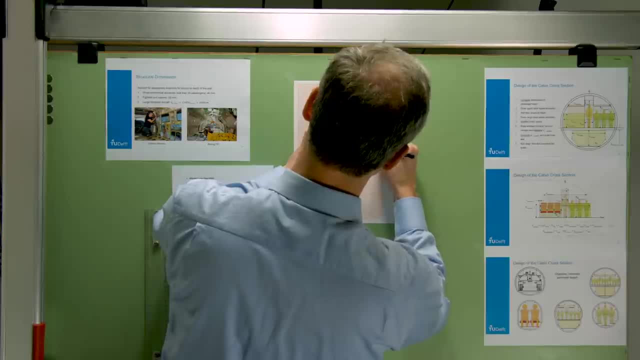 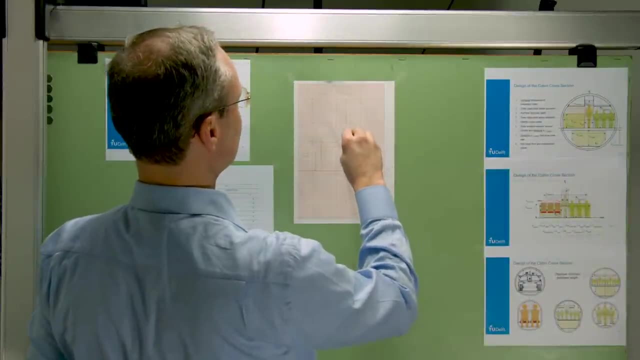 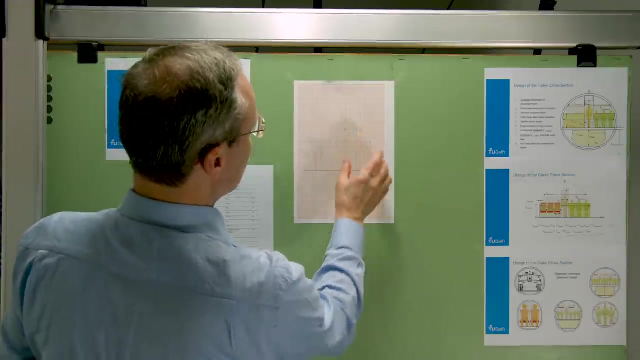 Again draw a straight line And then again you see you have immediately a problem. What's wrong here? What's wrong here is that you now aim at this highest point, but it's the width of this whole row of seats that is probably more limiting. 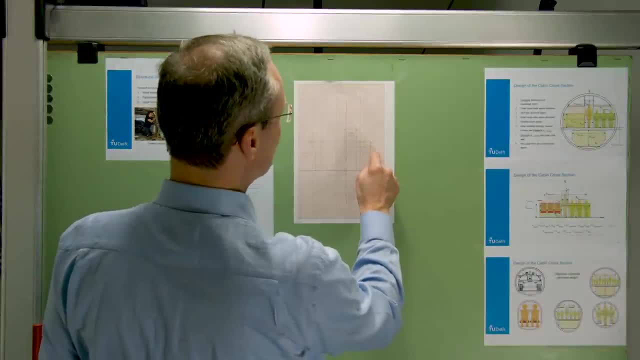 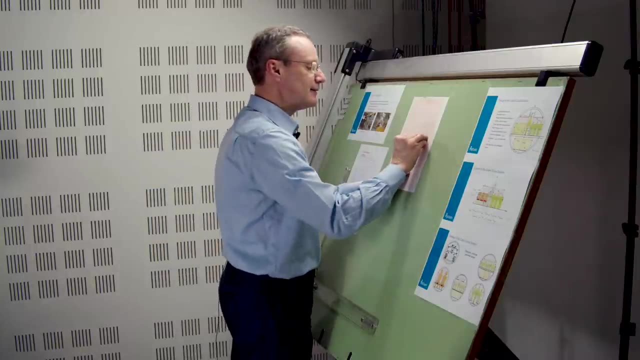 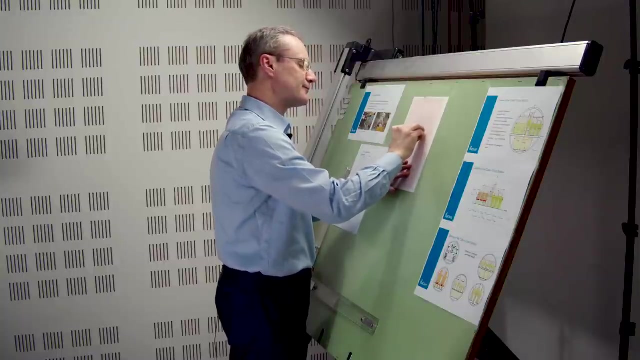 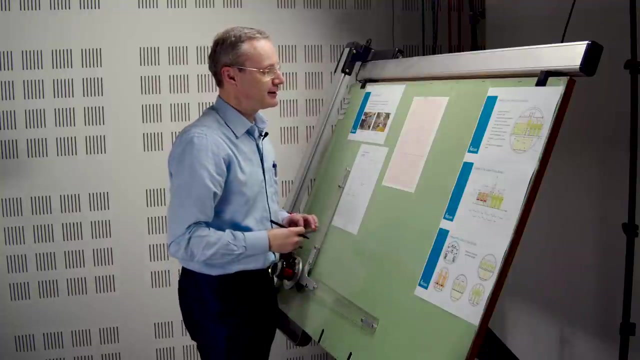 So you need to probably aim for this point and this point, or this point and this point. So let's do so Again. remove the line here. You can also remove the auxiliary line there- And let's apply the trick again. Let's say, okay, 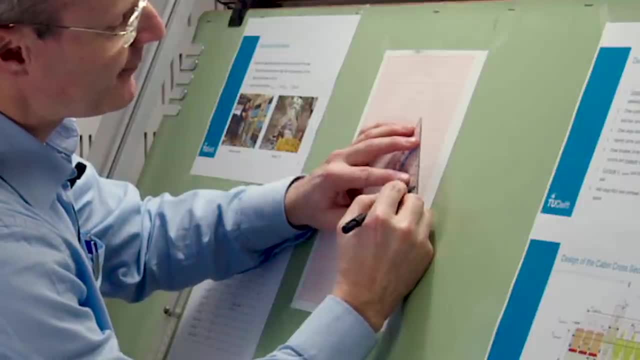 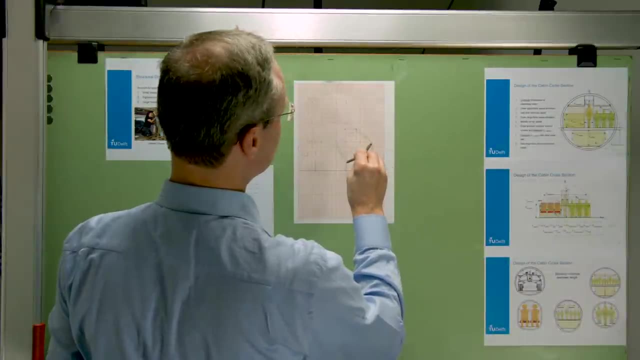 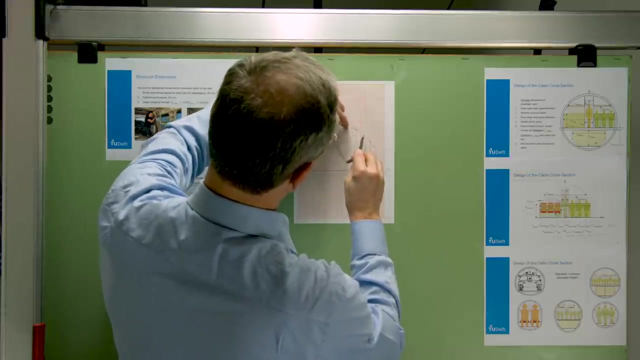 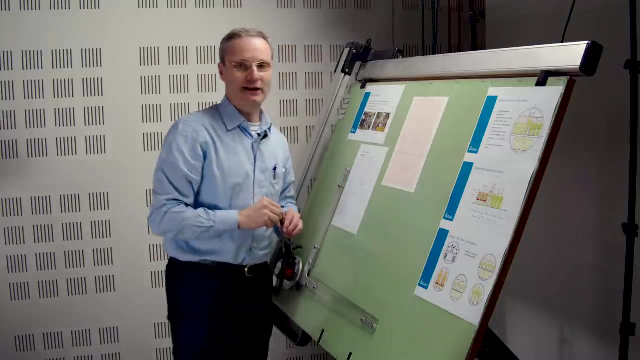 now expect that these two points will be limiting. Again, you see that this is not a solution. You will be out of the corner points here, But all the other ones, they are okay. So we, slowly but steadily, are getting there, And again, this is requiring some trial and error. 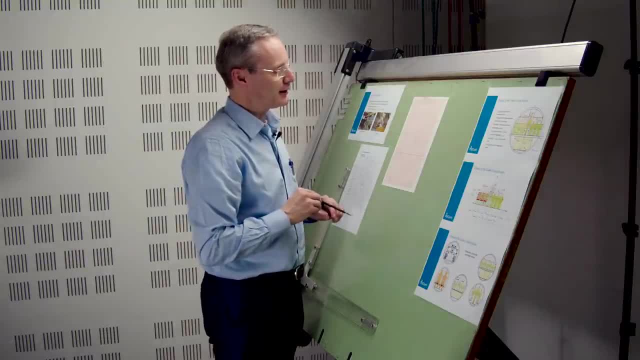 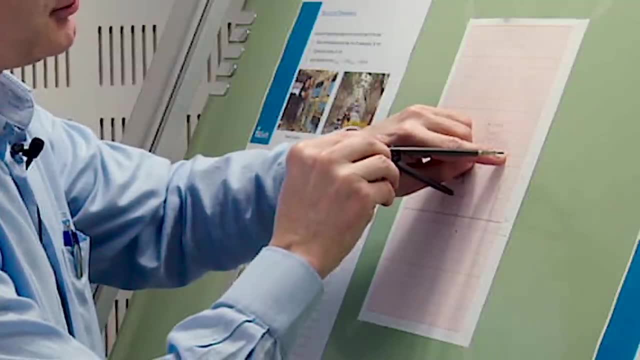 to find the nicest solution. So we have to take into account that this point might be limiting. This point will probably not be that limiting, but maybe this one will be limiting. So let's see if we find a combination between these two. 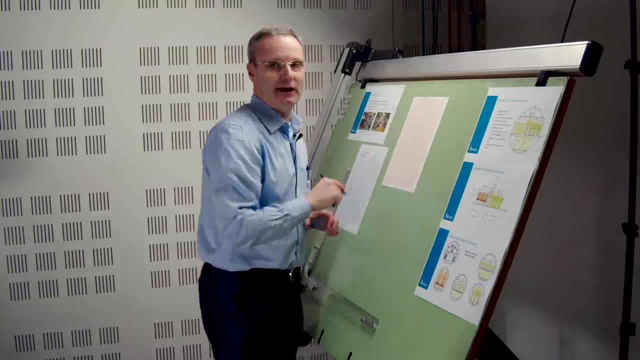 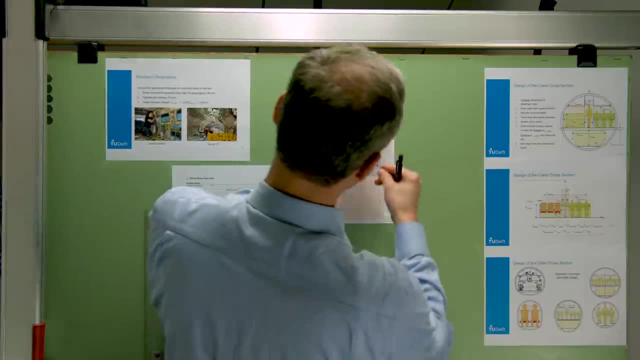 In this case, you see that I'm skipping the point, And you can do that because you will have a circle and that circle will be going around this point. So we can skip that point and we can make the line between these two points. 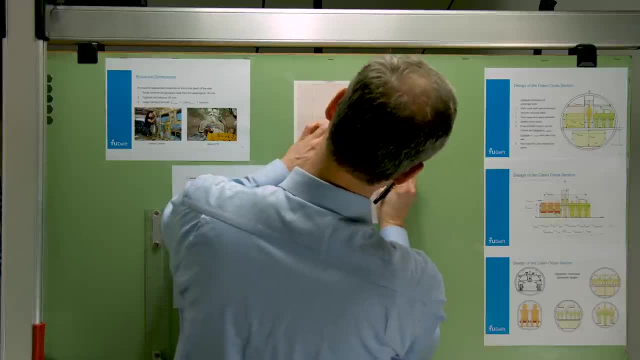 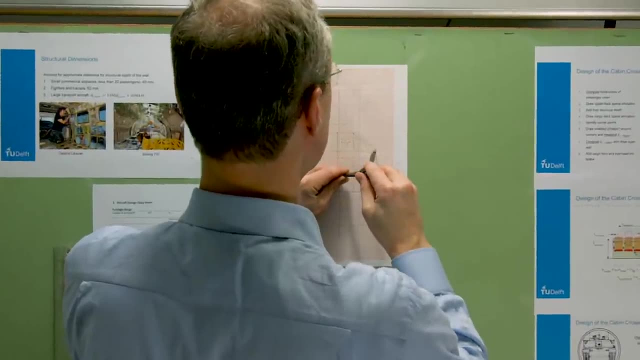 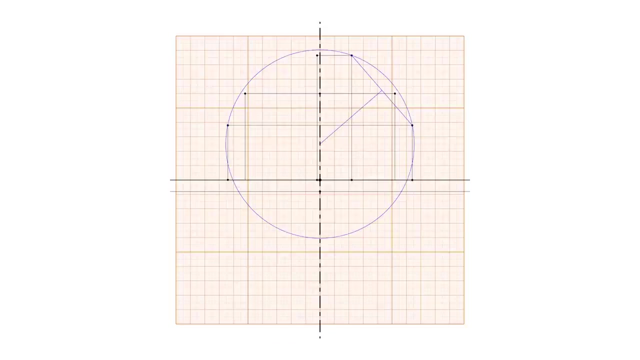 hoping that this will be enough, And then find these points, And you see, it nicely goes around there. Ah and there we have a new surprise. Now it looks like everything is okay, But we'll see that we are in trouble at this point. 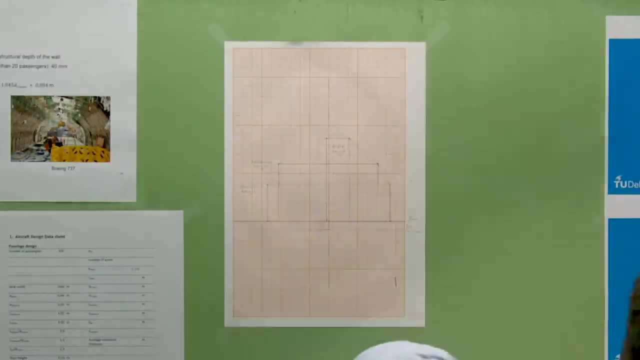 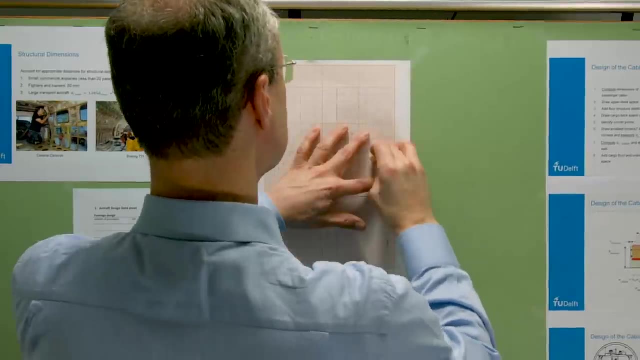 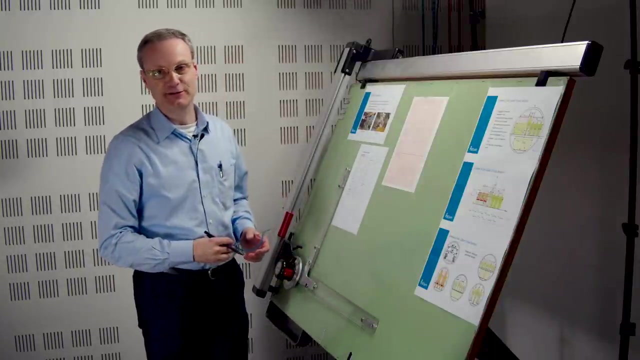 So it's even going to be more complicated, And this is a whole iterative process. you just have to go through to see what is the problem. So you need to take into account this point as well, And you have to find the most critical combination. 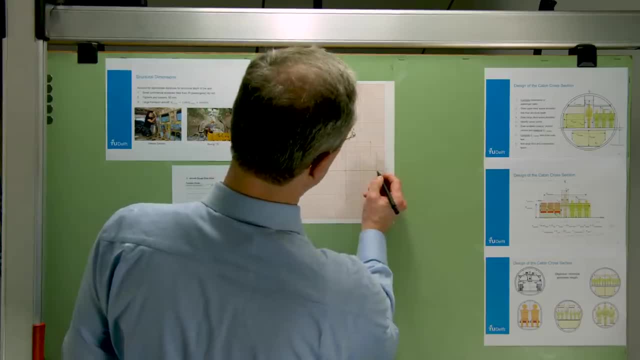 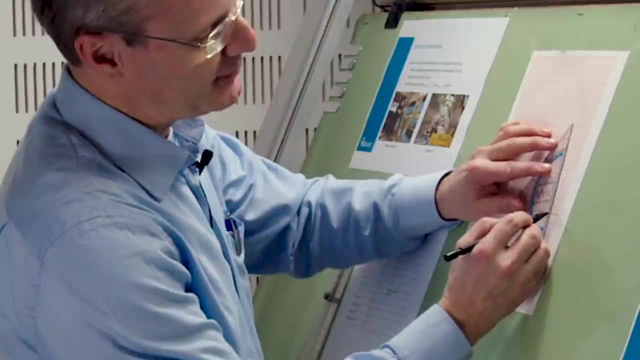 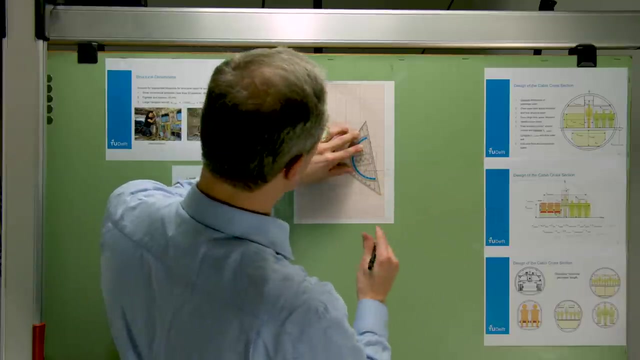 So it probably makes sense to start looking a little bit at what might be critical combinations. It might be that it's these two points. It might be that it's these two points, Then hoping that by the circle this point will be within the circle. 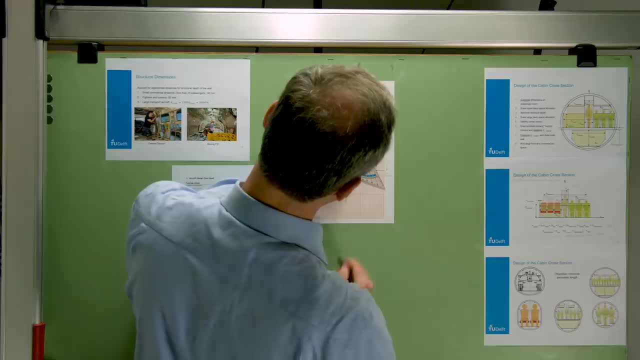 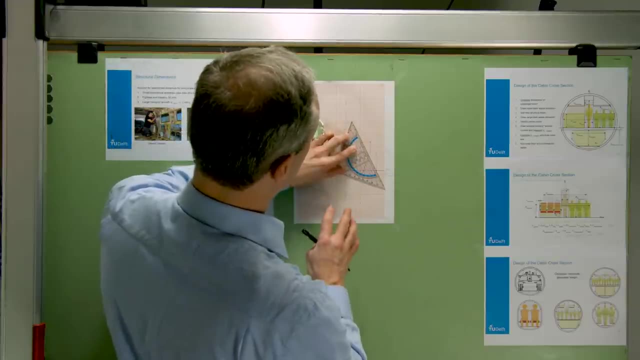 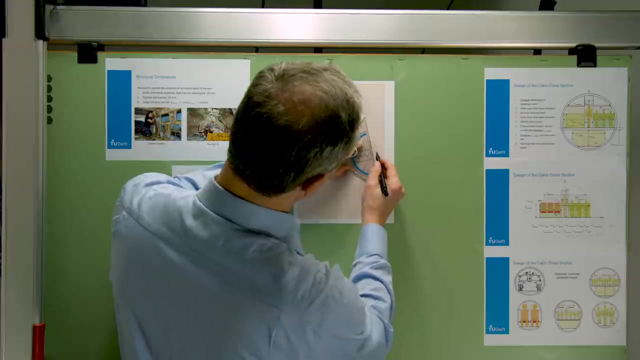 Or it may be these two points. Now, you see, if I take these two points, these points are pretty far outside of the intended circle. So that's probably not the right combination And it's doubtful whether, if you take these two points, this one will be within the circle. 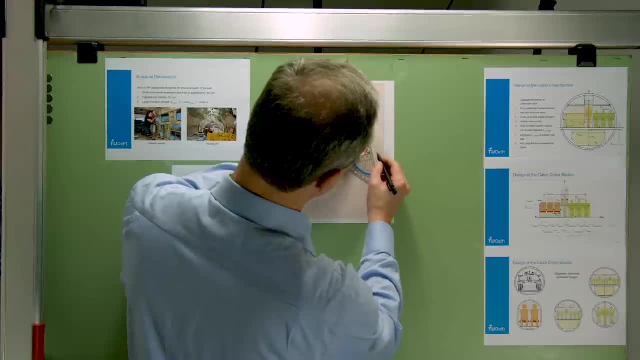 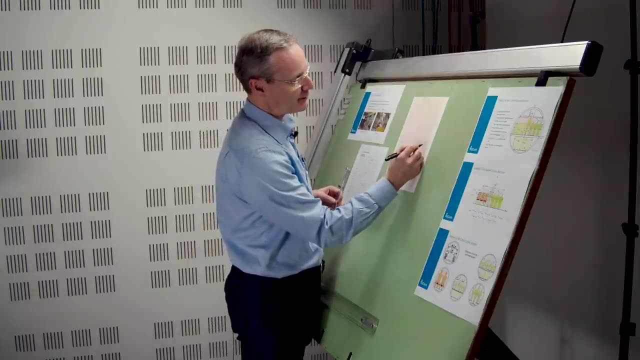 So my guess is that we have to take into account these two points and then make the circle around that. So let's try that. In this case it is already indicated by a line. So let's try that In this case it is already indicated by a line. 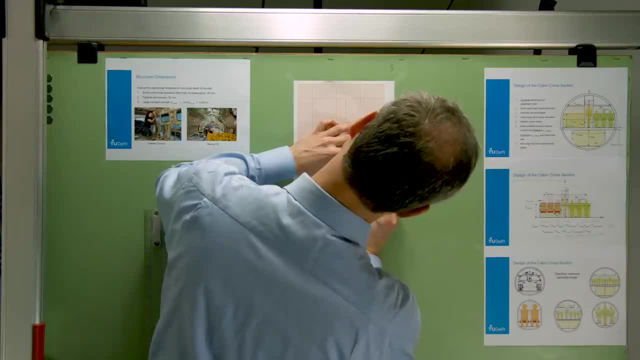 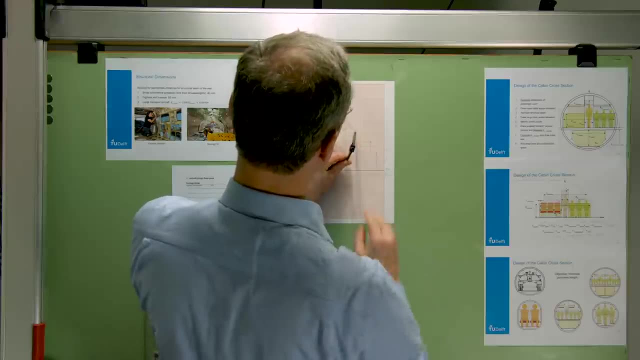 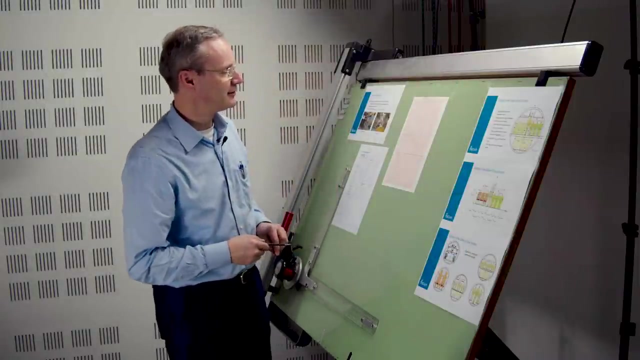 so we just have to find the middle of that line. This one is exactly in, And then you see this one is not going to be in. So again, this combination is not correct, So we have to find another solution for that. The tricky thing here is that you have 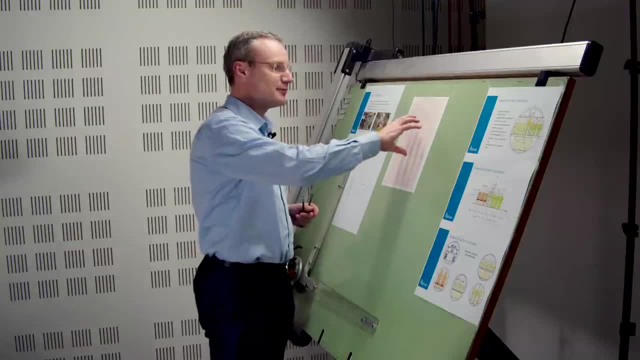 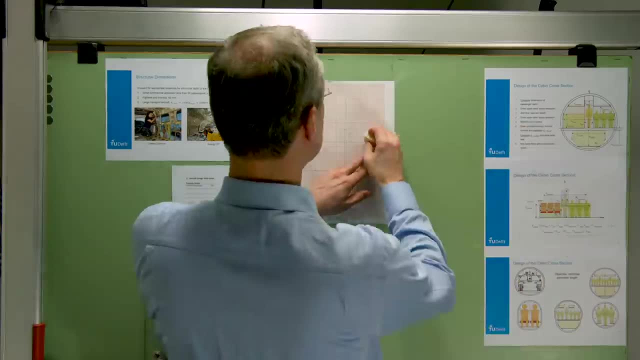 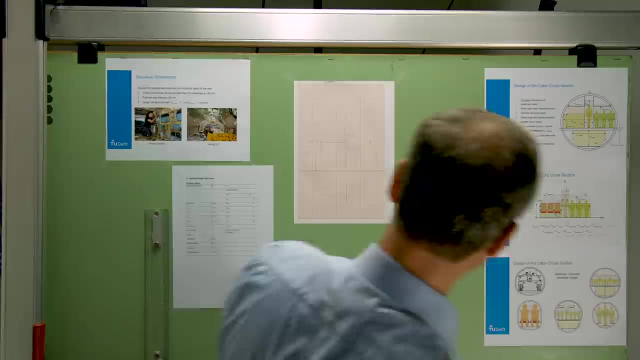 an asymmetric fuselage cross-section. So the fact that this is not symmetric makes life a bit harder for us, But let's just try to solve the problem. solve the problem, solve the problem. Okay, Let's try to get an indication first. 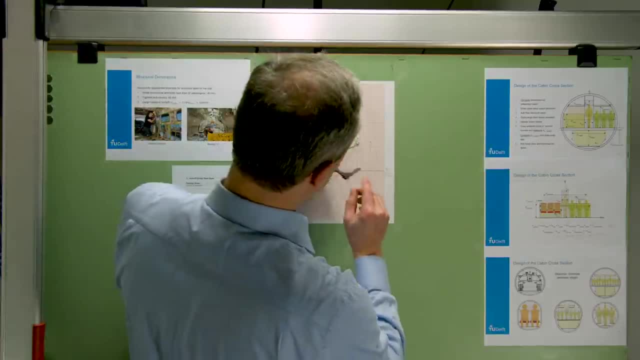 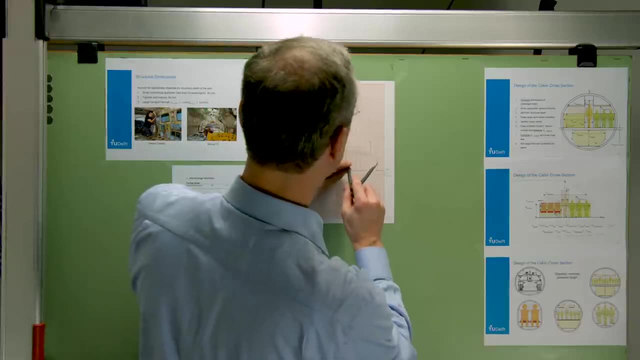 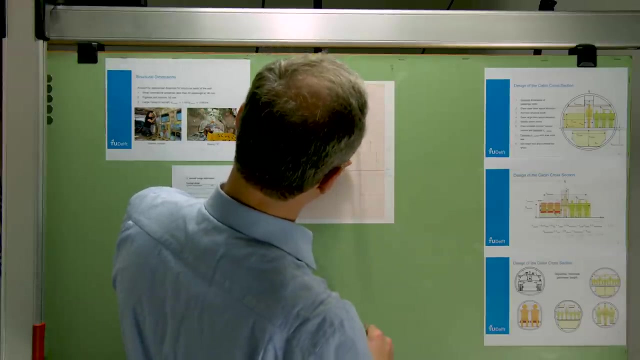 on how critical things are going to be. Suppose we take this point, this point, then we see that's not enough. Then we have a problem there, Because then we saw that this point is going to be tricky, that this point is going to be tricky. 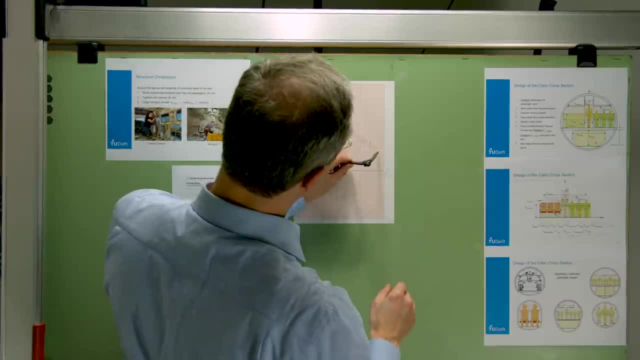 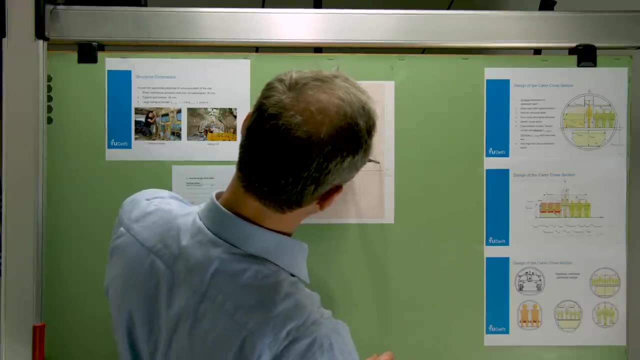 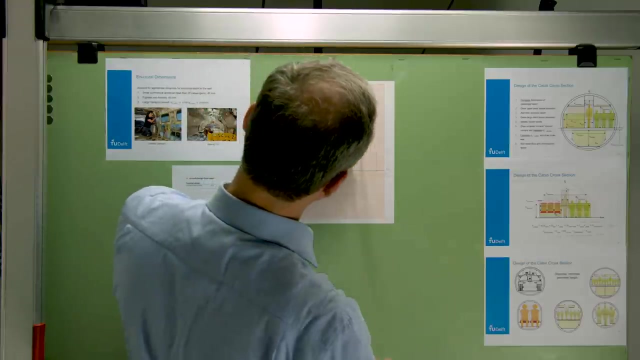 So maybe we need to take into account this point and this point And you see, probably the other parts will be in And if you go around you see that probably the other side is going to be okay as well. So let's again take this point. 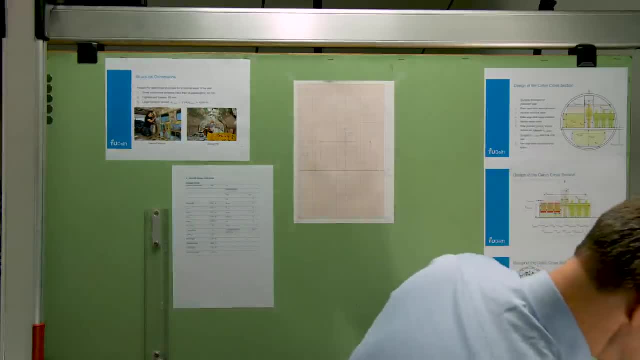 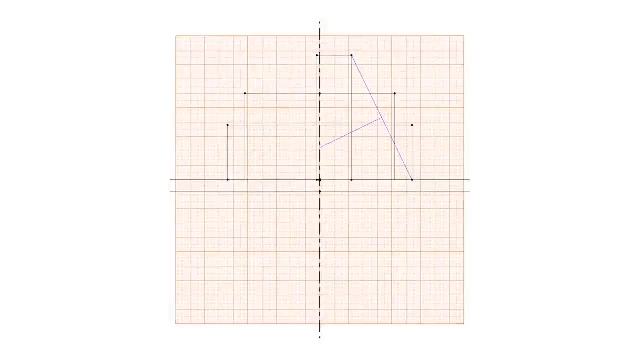 and let's take this point and see whether that's enough, and see whether that's enough, and see whether that's enough, And now we'll see that everything will work out. And now we'll see that everything will work out. And now we'll see that everything will work out. 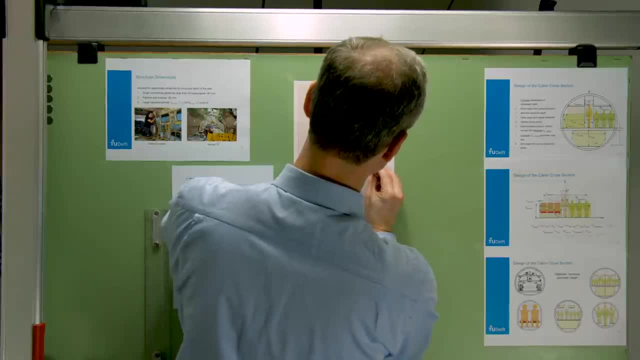 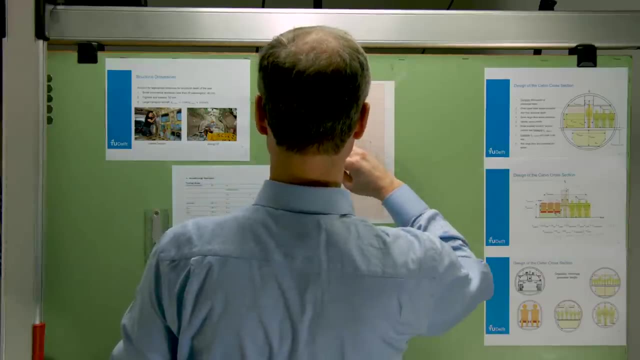 I have to nicely align this, I have to nicely align this, Going around touching that point free from the other point, And here we have our circle at last. And here we have our circle at last. So this can be a rather tricky process. 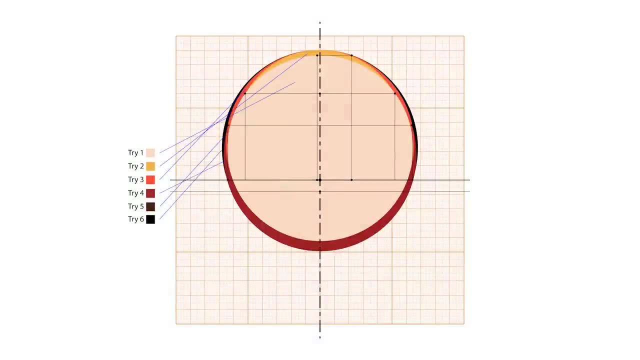 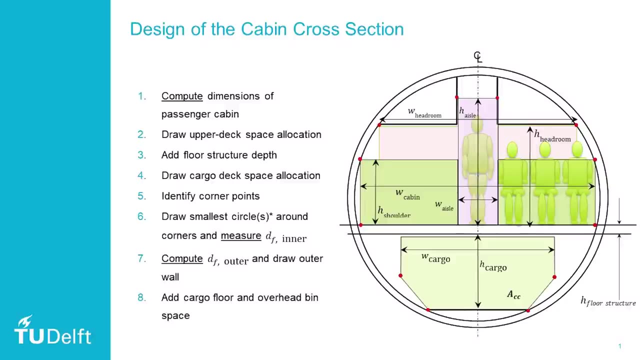 This will take some time, normally, But now we're there. So what we've done? we have computed the dimensions. we have the upper deck, we have the upper deck structure. In this case it was not relevant, We had no cargo. 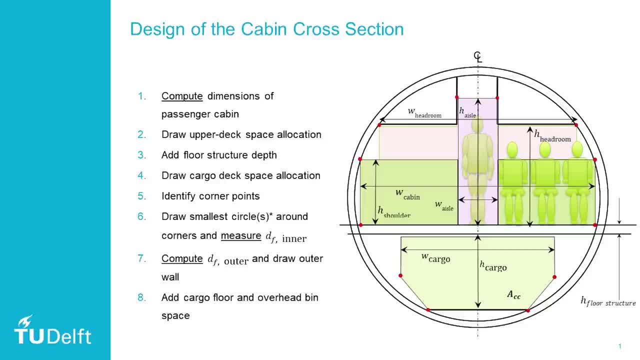 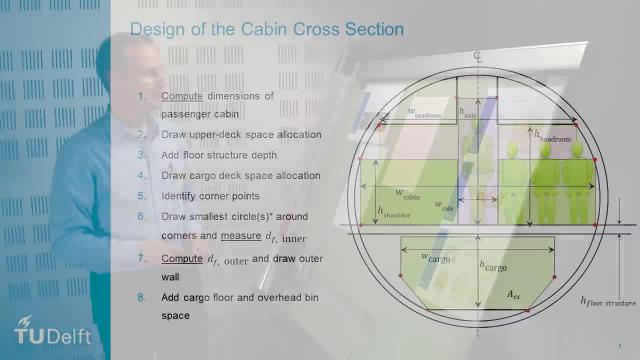 some lower deck situation. We had a corner point. We have now drawn the smallest circle around it And then the next step is measure the inner diameter of the fuselage. measure the inner diameter of the fuselage. In this case we have an asymmetric. 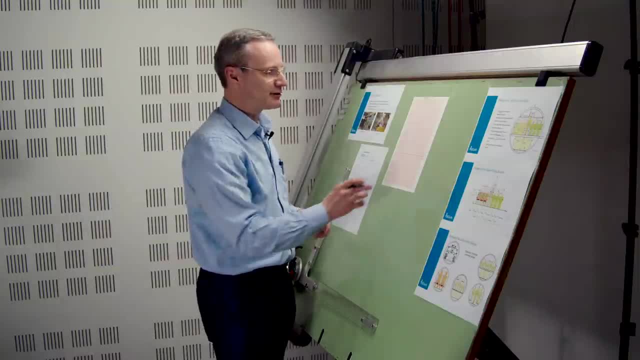 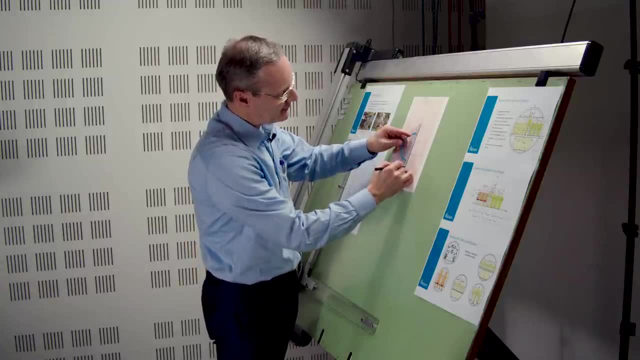 division of the seats here, So it's a bit tricky to figure out where exactly is the other center line, But the best way to do this is to make use of the center line that has already been given here. So make use of the vertical center line. 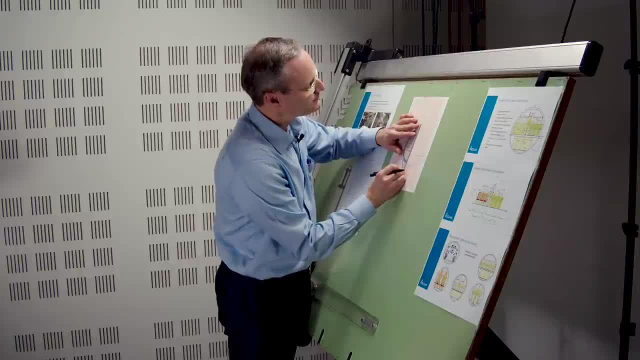 to measure it. I'm going to use my protector again. I'm going to add this to the top point. I'm going to add this to the top point. That is going to be like this, And then my bottom point is here: 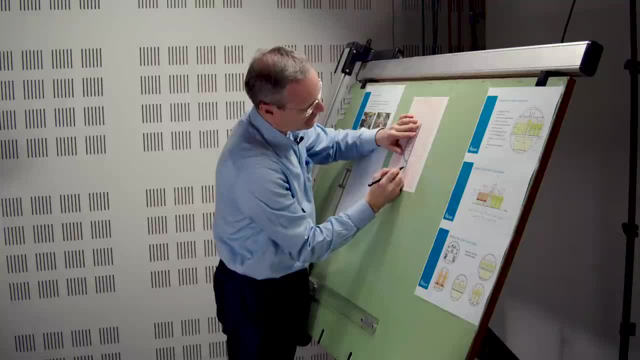 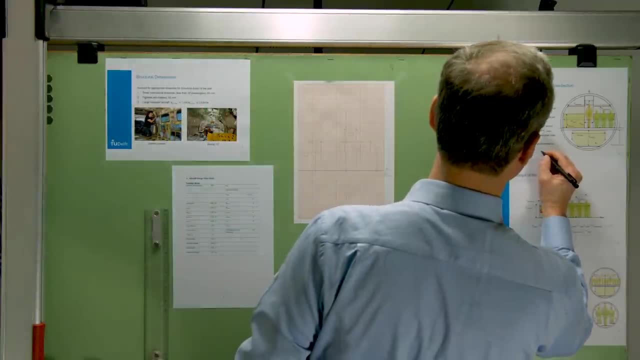 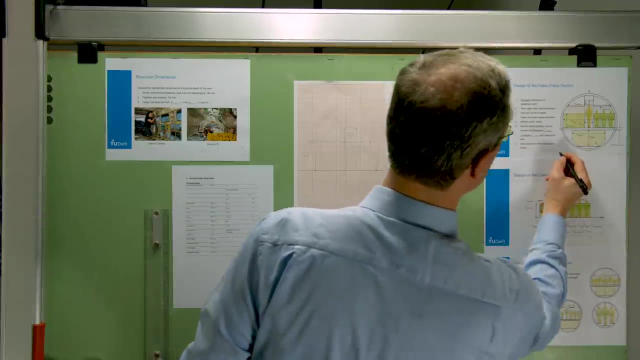 That means I have 7 centimeters plus 6.6.. So we have 13 centimeters plus 6.6 centimeters And we need to multiply this by 25 because we have the scale of 1 to 25.. the scale of 1 to 25.. 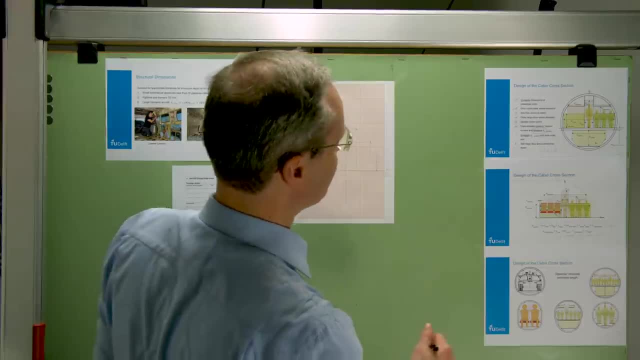 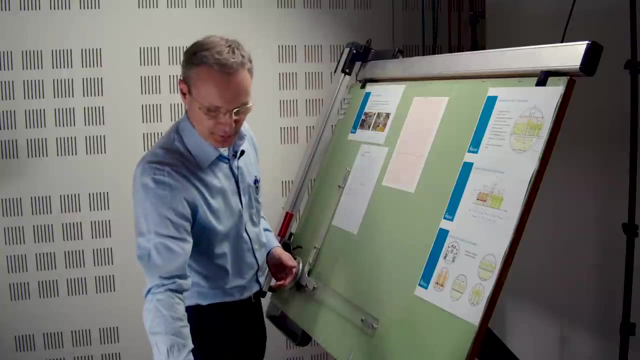 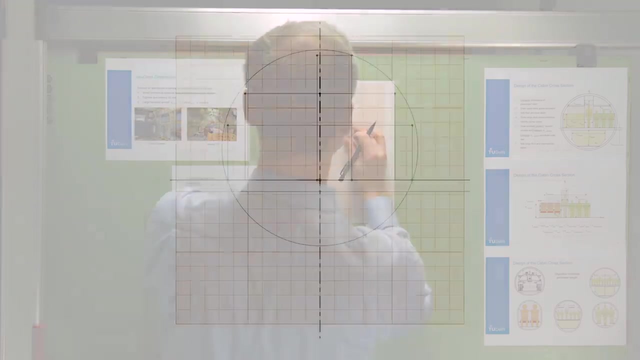 We have 13.6 times 25.. We have 13.6 times 25.. That gives me 3.4 meters. 3.4 meters is going to be my inner fuselage diameter And I can draw that in the diagram. 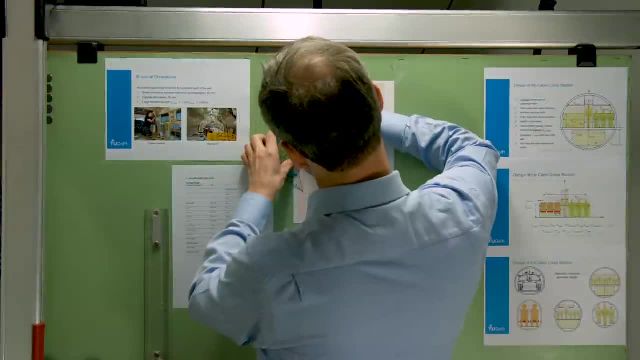 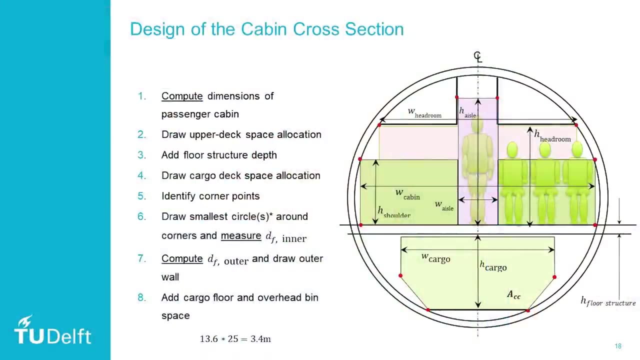 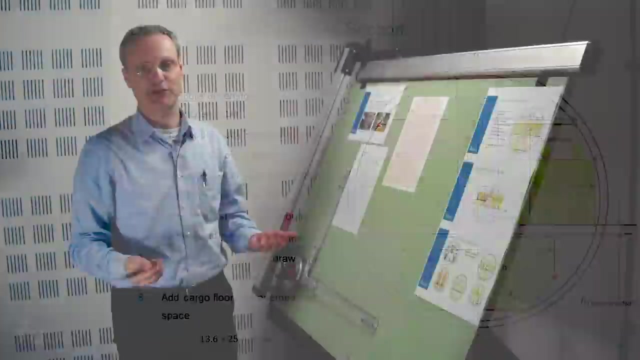 And I can draw that in the diagram. And I can draw that in the diagram. So the primary dimension is going to be 3.4 meters. Okay, Step 6 done. Now. Step 7 says: compute the outer diameter and draw the outer wall. 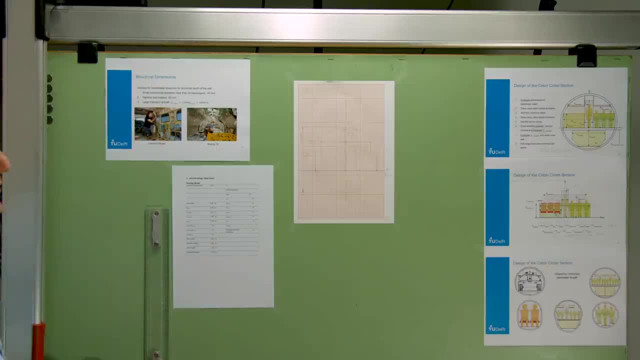 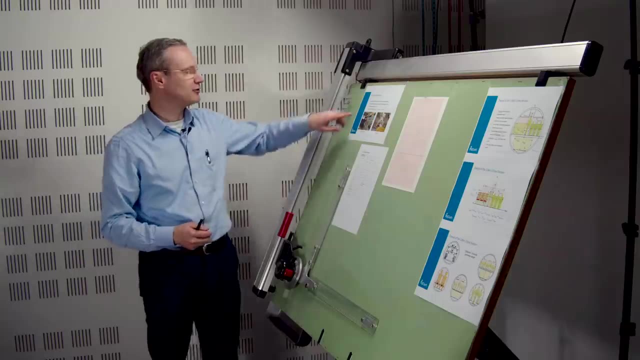 How do we need to do that? Well, we need to go to this slide, the structural dimensions. We do have the structural dimension of the floor, because that has been given, But for the structural dimension of the wall we are going to use a small aircraft. 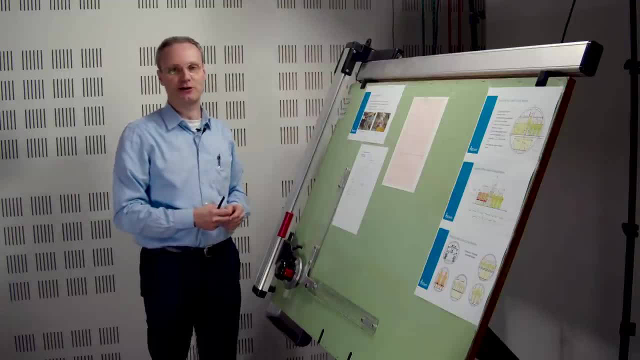 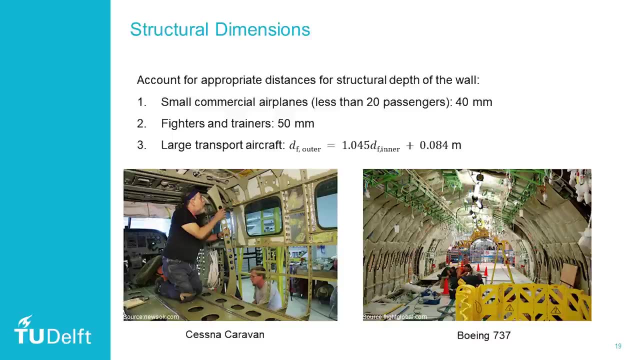 because this is not a fighter or a trainer and this is not a small commercial aircraft with 20 passengers. So we'll make use of this formula here, which says: it's 1.045. it's 1.045 times the dimension, and we use meters here. 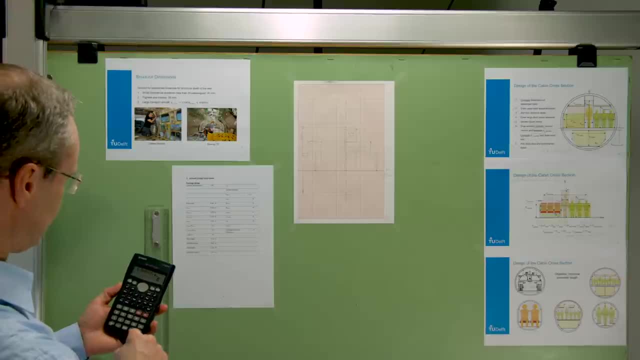 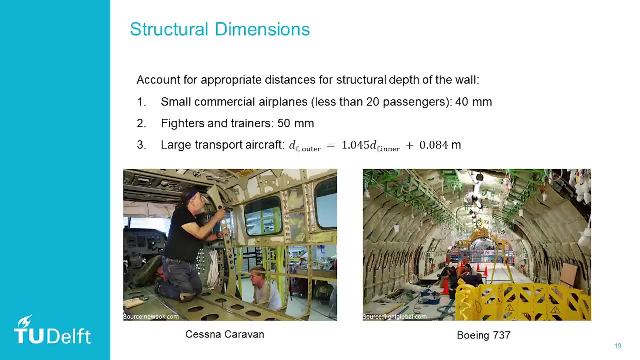 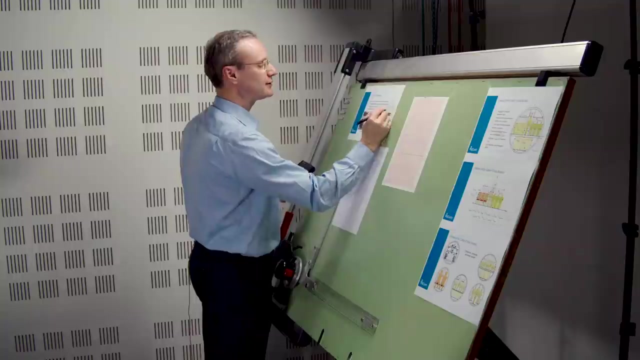 So 3.4 meters times 3.4 meters, times 3.4 meters, 8.5 centimeters, 0.084. So my outer diameter is going to be 3.59 meters, 3.59 meters, 3.59 meters. 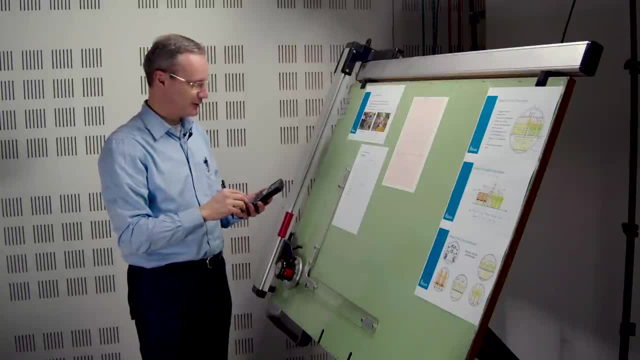 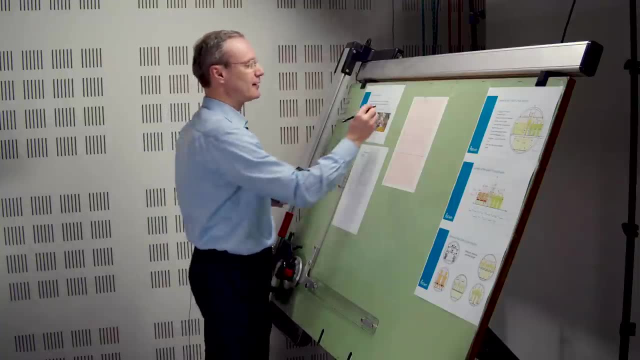 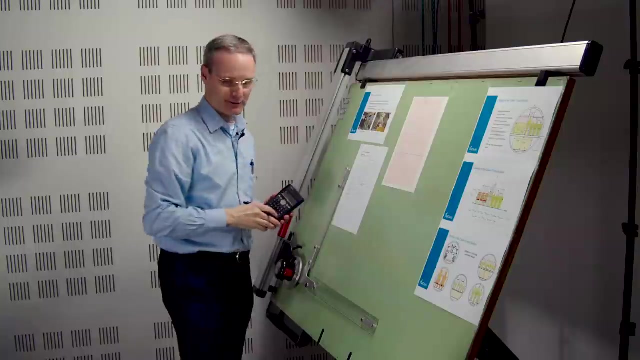 I have to again divide that by 25 to bring it back to the, to bring it back to the 359 divided by 25, to bring it back to the scale. so that leads me to 14.36 to 14.36 centimeters on the drawing. 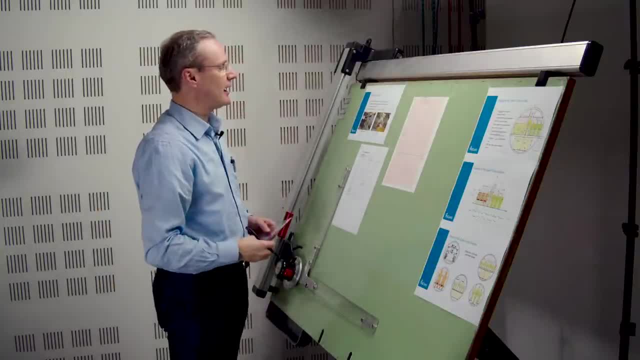 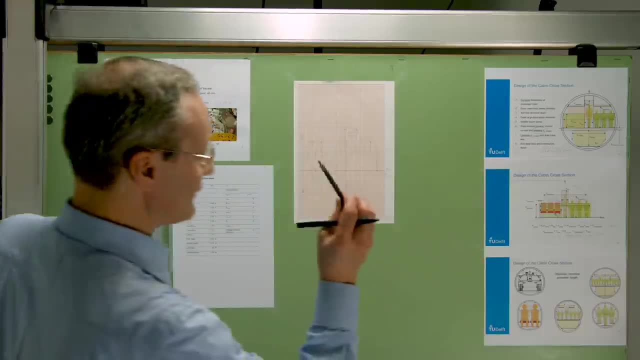 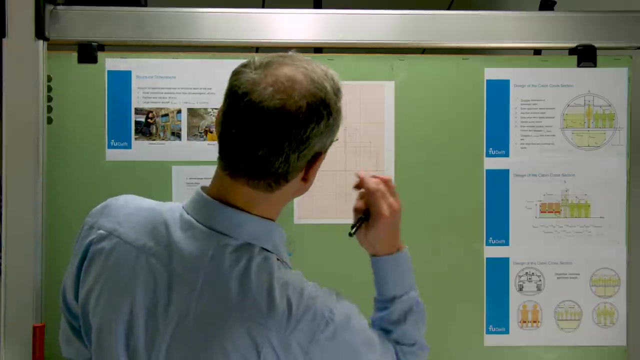 centimeters on the drawing. so that's what I'm going to do. I'm going to take half of it because I'm going to set the diameter using the compass. again, using the compass, again, I'm going to figure out how this dimension is there and what I'm going to do. 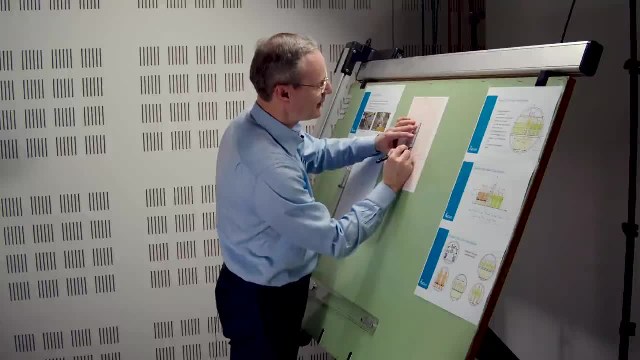 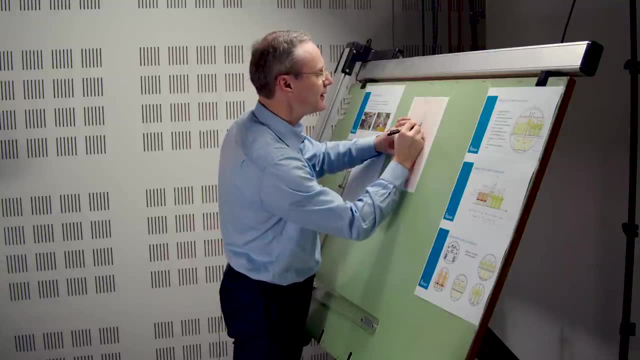 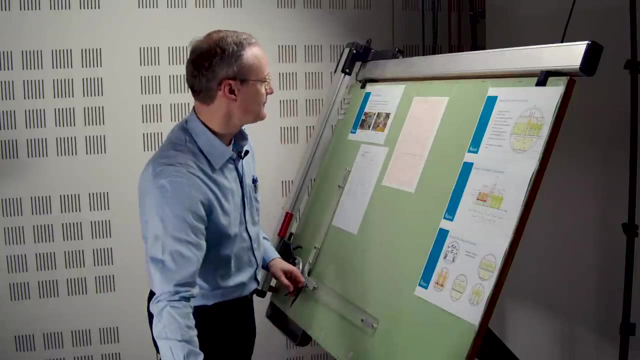 this was the center point and I'm going to make use of 7.2 millimeters, of 7.2 millimeters, and then I have to add 2 millimeters over here. this is going to be over here. I have my center line, my center point, over here. 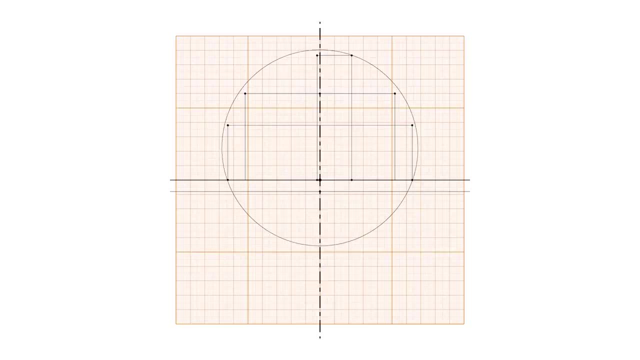 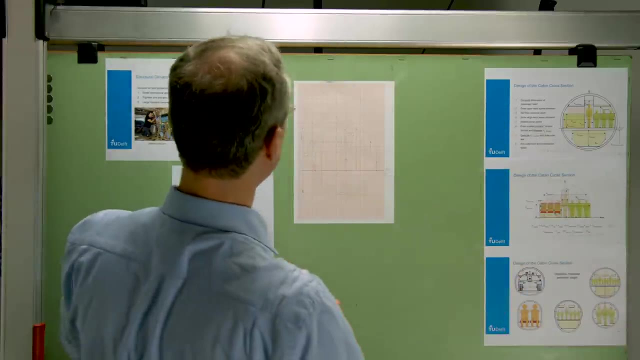 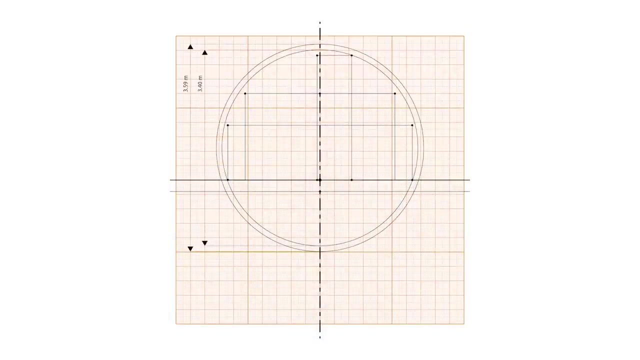 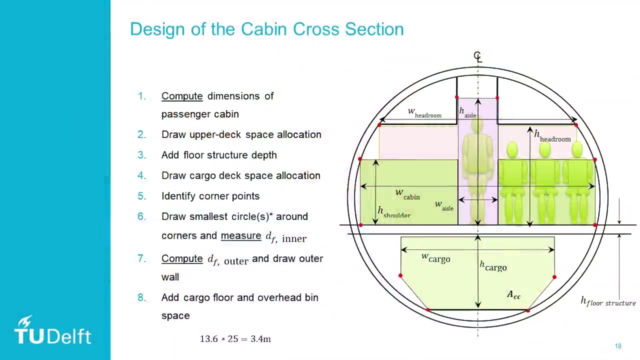 size this. so here I have my outer diameter, and the best way is to also indicate that dimension. so let's do that here. so I have computed that. I've drawn the outer wall, I've drawn the outer wall, and then step 8 is the cargo floor. 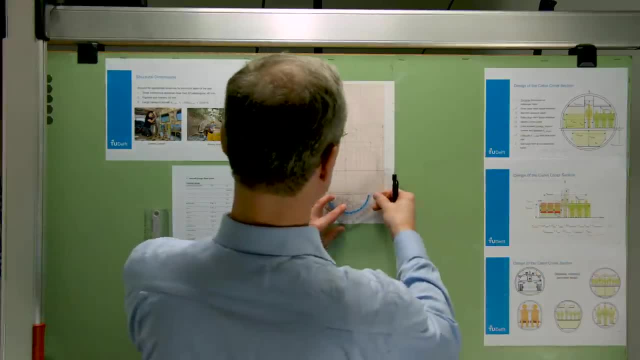 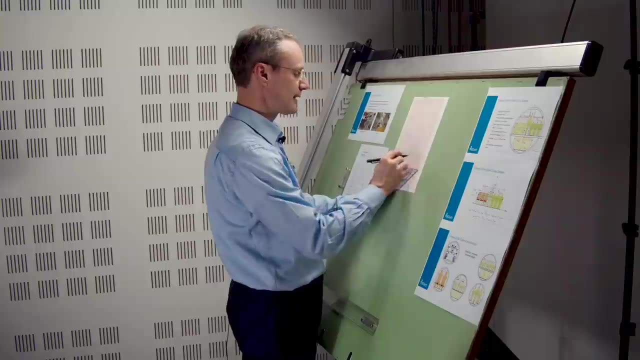 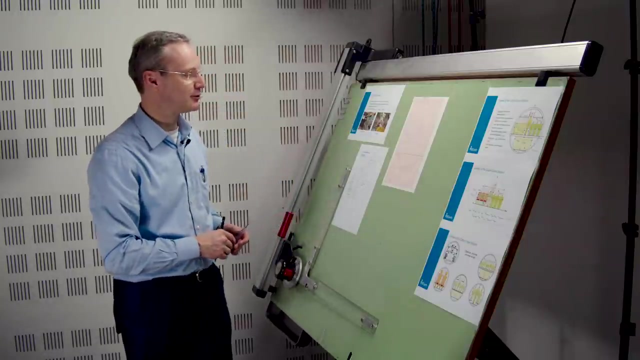 in this case there is nothing being given, but you could draw a cargo floor that could, for instance, be here, because the cargo will not be resting on the bottom of the structure. you probably want to feed some cabling through there or some ducting, so we can have a cargo floor here. 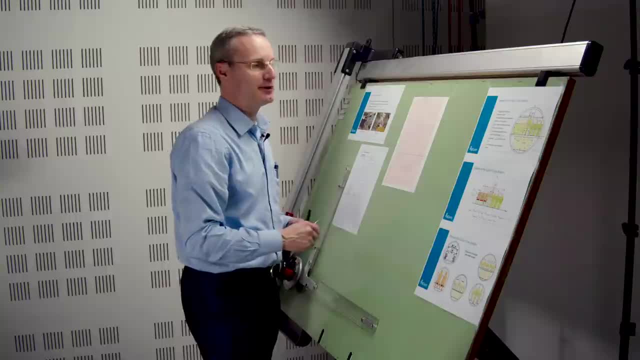 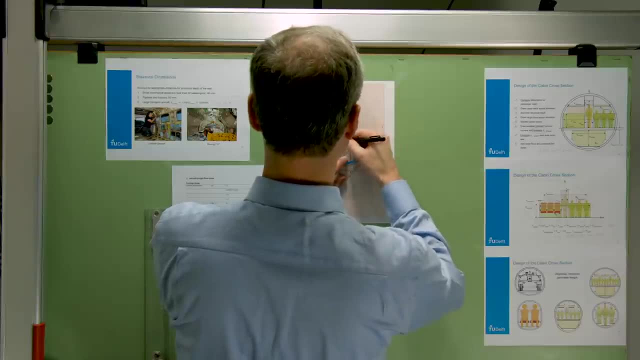 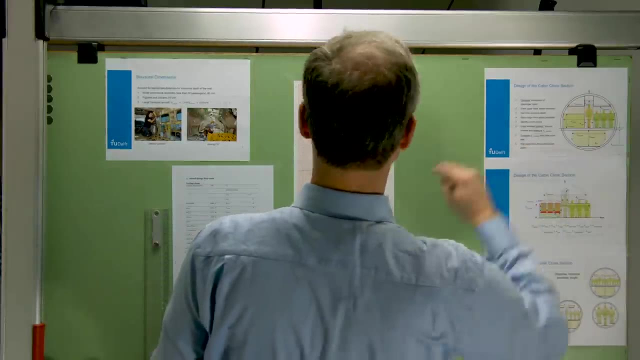 nothing has been given, so this is ok, and we can add overhead bin space in this case. let's make these lines a bit more clear in this drawing. so we know that this is the headroom space, so above that there will be the luggage bins. so in this case that's just going to be. 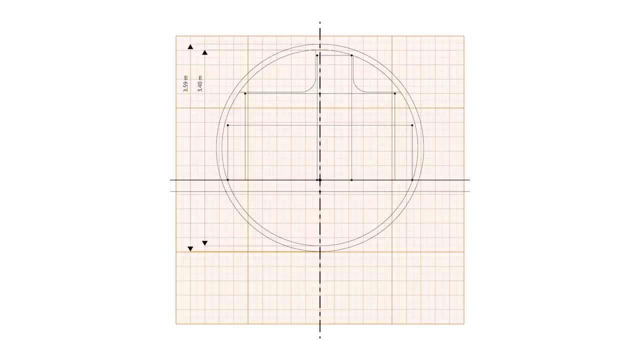 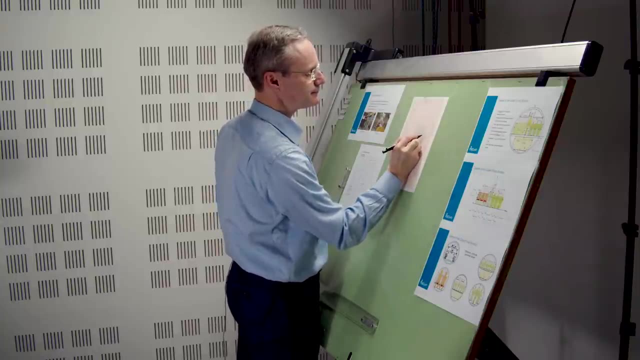 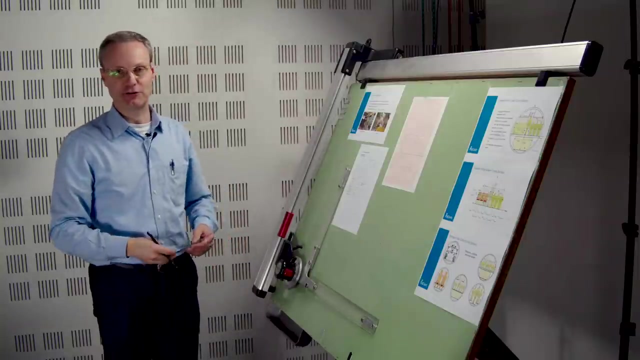 an artist impression that could be something like this on both sides of the aisle. and, of course, the modern aircraft. you would like to have the cargo bins as large as possible. so in a real aircraft you would have some dimension of suitcases you want to bring along.